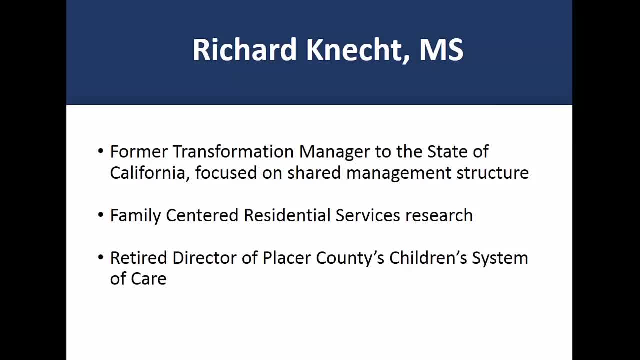 residential services and is a fellow of the CREA Center for Child Welfare and Human Services. Richard Kinect is a consultant and advisor to the Children's Health and Health Services and the Sierra Health Foundation's USC Marshall School of Health Leadership Program. He is the retired director of Placer County's highly regarded Children's System of Care. 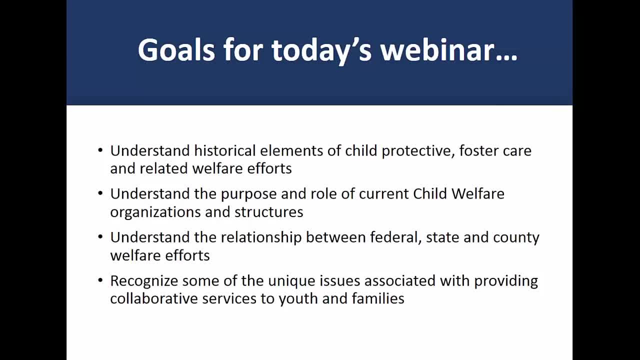 Thank you, Kim. It's nice to be with you today. We hope that this work will be useful to you as you work with CPS and child welfare partners in your community. As we go through our material, we hope at least four outcomes are possible for you today, One that you'll 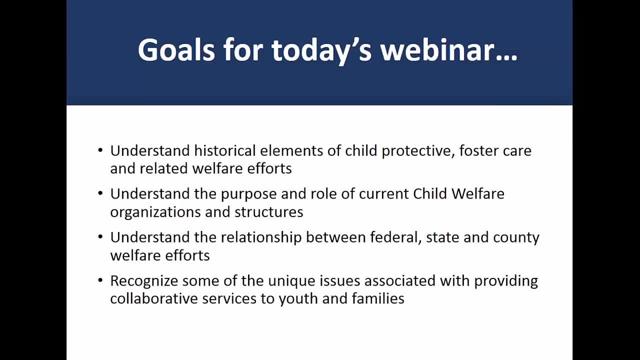 have an understanding of the historical elements of child welfare. Two, that you'll have an understanding of the structural elements of child welfare. Three, that you'll have an understanding of the scientific effects of child welfare on individuals of all ages, programs, children and all families. Four, that you'll have an understanding of the role of him in this work, including child protection, foster care and related welfare efforts. Five: that you'll have an increased understanding for the purpose and role of welfare efforts in your community and the structures which support them. Six: that you'll 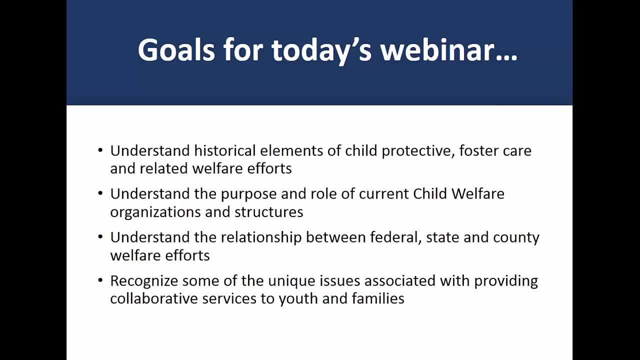 have an understanding of the relationship between federal, state and county welfare efforts. Seven, that you'll have a recognition about some of the unique issues associated with providing collaborative services to youth and families. We are indebted to two sources of information for our webinar content today. Much of the 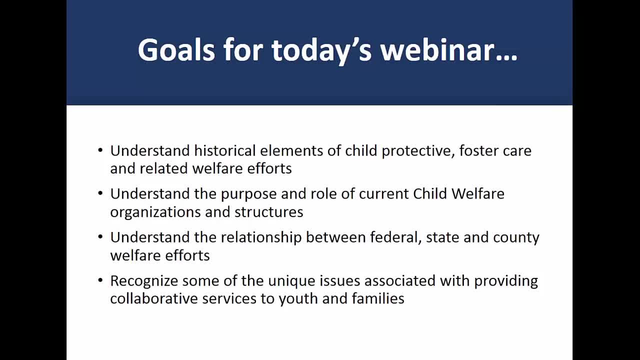 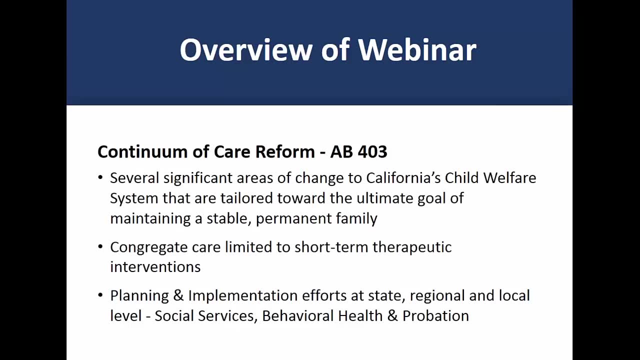 information is from the Child Welfare Information Gateway and its parent funder, the US Department Health and Human Services Children's Bureau, and secondarily from the California Center for Research on Women and Families. The effort known as the continuum of care reform draws together a series of existing and new reforms to 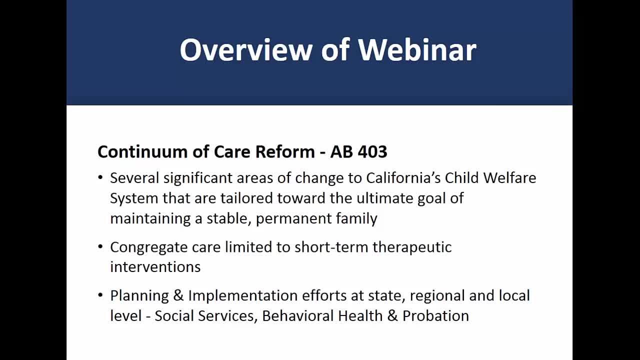 the state's child welfare services program, designed out of an understanding that children who must live apart from their biological parents do best when they are cared for. in committed to nurturing family homes, Assembly Bill 403 provides the statutory and policy framework to ensure services and supports provided to the child or youth and his or her family are tailored. 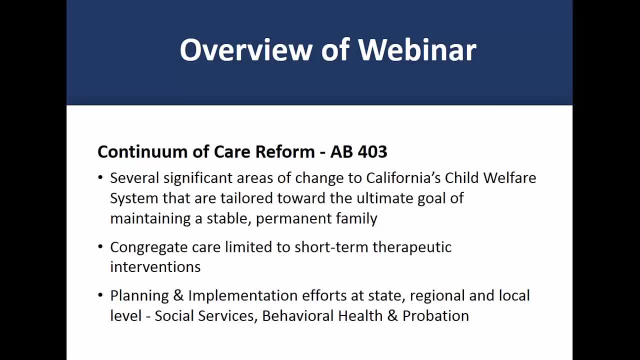 toward the ultimate goal of maintaining a stable, permanent family and reducing trauma on all involved. Reliance on congregate care should be limited to short-term therapeutic interventions that are just one part of a continuum of care available for children, youth and young adults. While Assembly Bill 403 is 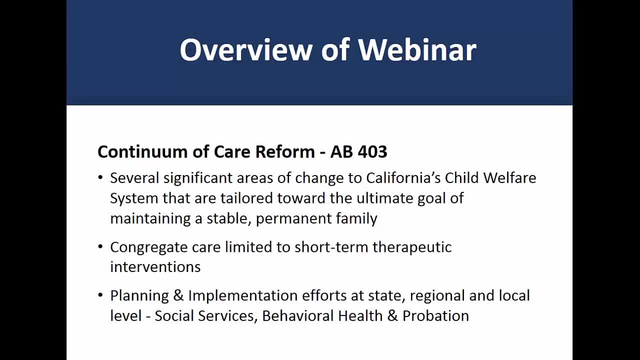 a wonderfully designed piece of legislation, it does create challenges for state and county implementation efforts. As part of CIBHS efforts to work with DHCS around CCR, CIBHS has developed this webinar for behavioral health care systems. The webinar is focused on providing an 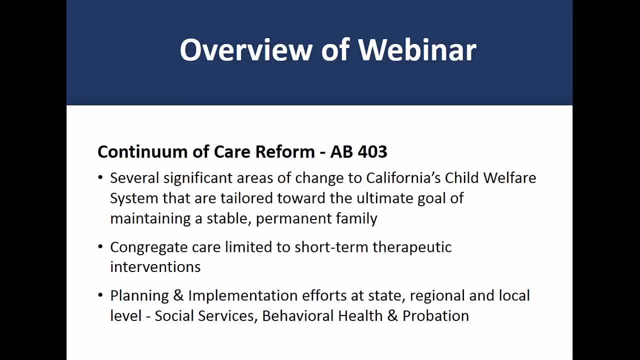 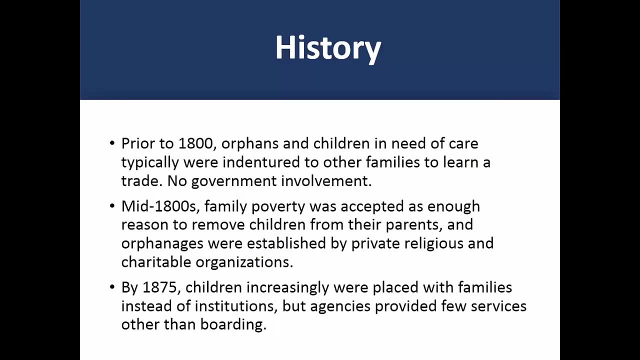 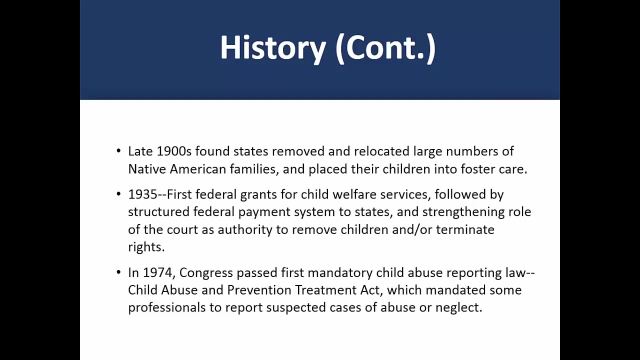 overview and purpose of California's child welfare system. We recognize that many county child welfare and behavioral health systems are already collaborating and working together. Let's begin with a short look at the history of child protection and intervention. Before the 19th century, there was no public authority or involvement in 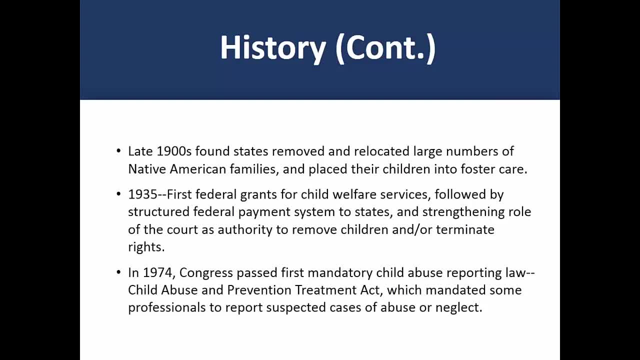 protecting or ameliorating neglect and abuse. Some of the more zealous groups removed children from their homes, with little regard for parental rights, and there was no court oversight. By mid-century, awareness had grown about what constituted child neglect and faith-based systems often mobilized. 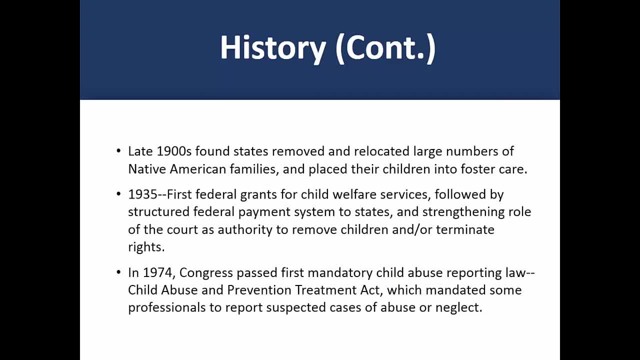 without government involvement to protect children. Some of these agencies practicing early child abuse and child abuse prevention still are available on the East Coast and function as Children's Aid Societies. Like all providers, they've evolved and adapted their care models and today are active and involved partners in foster. 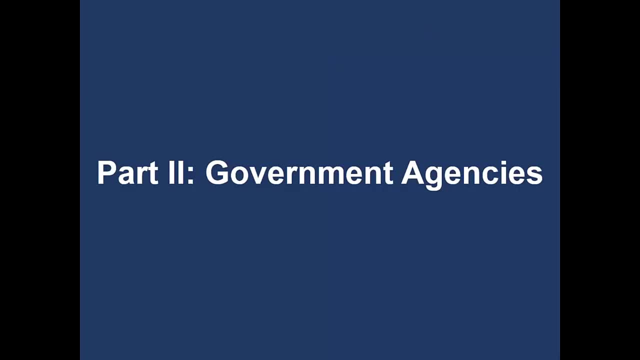 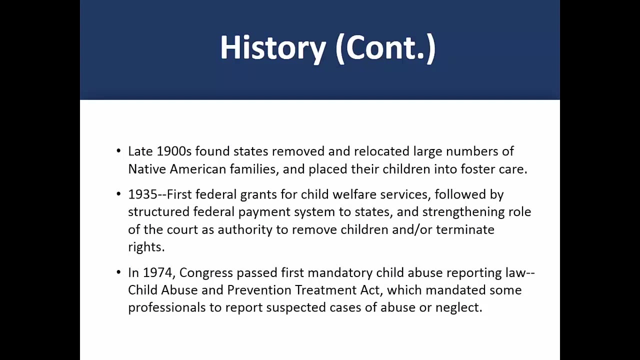 care services delivery. By the late 20th century, federal and state laws existed and were sometimes implemented inconsistently. Perhaps the most egregious example is the use of the federal and state laws. The federal and state laws were introduced in the 19th century. The federal and state laws were introduced in the 19th century and were: 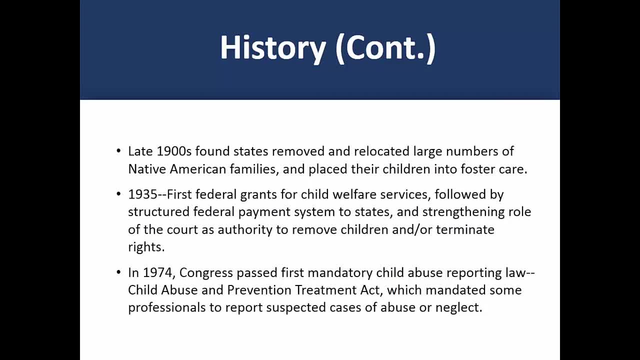 actively being introduced by the government, having been adapted and manipulated within the area of foster care and then capitalized on state authentication practices. so the federal and state laws were used over account for the use of the federal legislature. A Bundley頓 is the relocation of large numbers of Native families, Perhaps sorry. they were relocated for reasons not for abuse and neglect, but out of belief that children be better served. in, I'm meant ev of home. This is known, of course, as the Trail of Tears. The first real funding of child welfare efforts began around 1935 and links the state's involvement to court systems for independent oversight. The late 1930s involved in the toma branch and the CPSI sini. 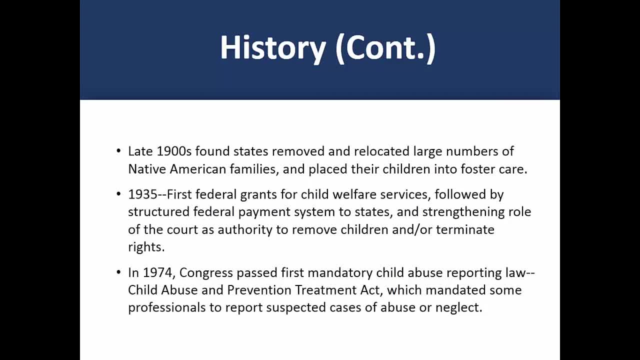 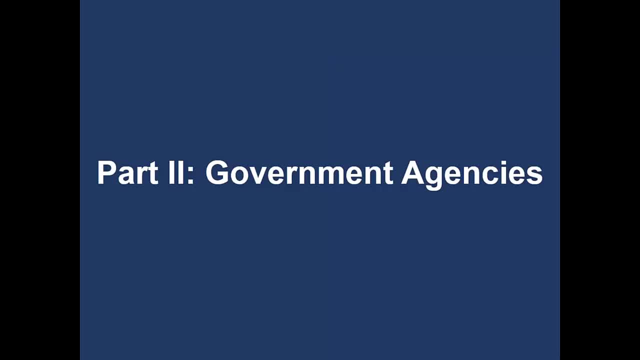 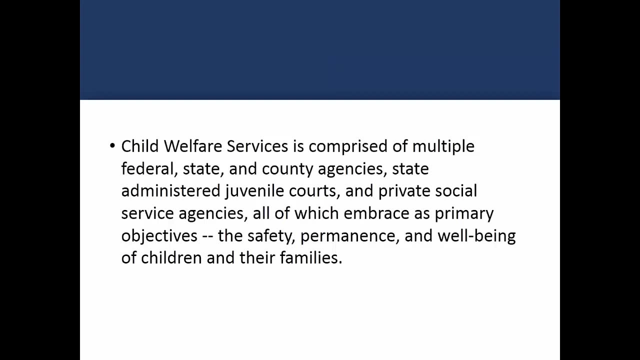 I standsточmenna. It wasn't until 1974 that the first mandatory abuse reporting laws began in this country. There are three levels of government support and oversight to the delivery of child protection and foster care services. Federal and state laws establish the legal, regulatory and fiscal frameworks that govern. 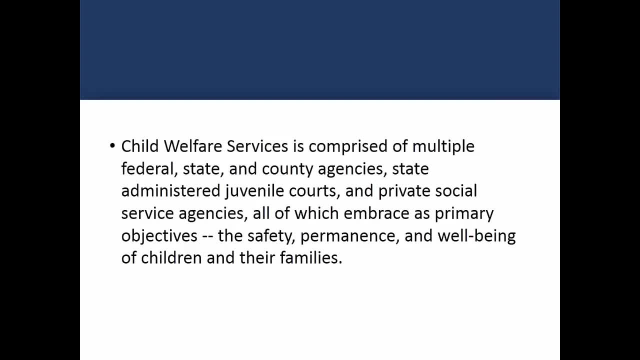 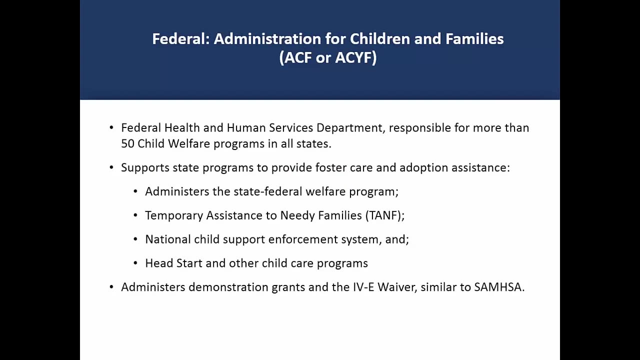 the roles and responsibilities of agencies and organizations for children and families that enter and leave the child welfare system. There are now nationally recognized goals for all child welfare systems, focused on safety, permanence and well-being. The federal government itself is a complex organization and uses various vehicles to 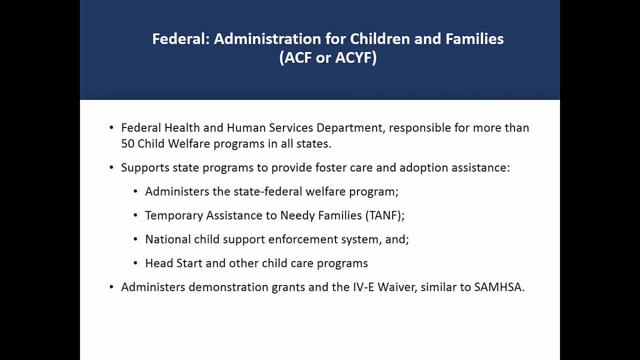 fund child welfare. Each of the four programs listed here is intended to assist state, county, city and tribal governments and public and private local agencies to provide services through funding allocations, policy direction and informational services, Known also as the Children's Bureau. the federal authority funds a number of programs. 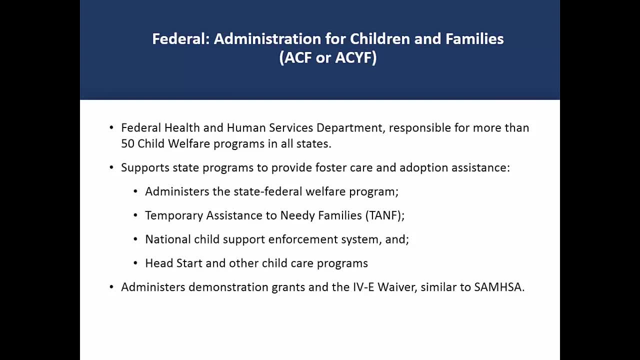 that focus on preventing abuse and finding permanent placements for children who cannot safely return to their homes, and supporting independent living program services for youth who will or have left the foster care system. The Children's Bureau also supports system improvements through a series of national resource centers, regional implementation centers and discretionary demonstration grants. 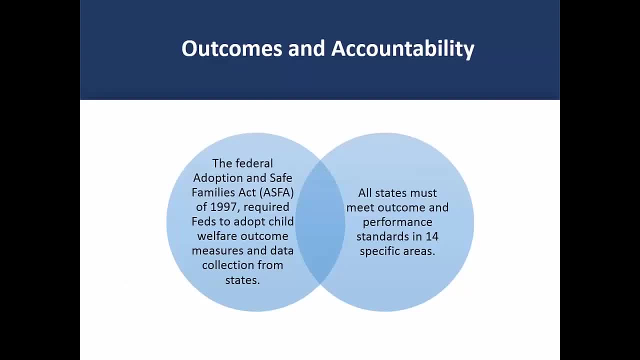 to states, counties and communities. Thank you. The federal administration offices have a significant role in building accountability in child welfare. Prior to 1997, there was little data-based or outcome monitoring. Today there are seven large outcome areas and each of those has a number of sub-elements. 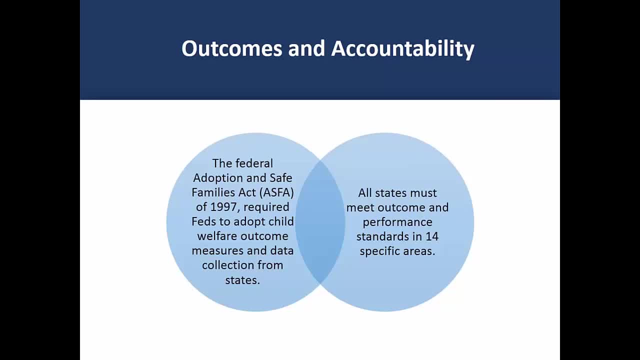 A couple of examples might include monitoring the reduction of recurrence of child abuse or neglect, seeking a reduction in the time in foster care to reunification without increasing reentry and, of course, monitoring placement stability. In California, counties can access a statewide clearinghouse known as Safe Measures to get 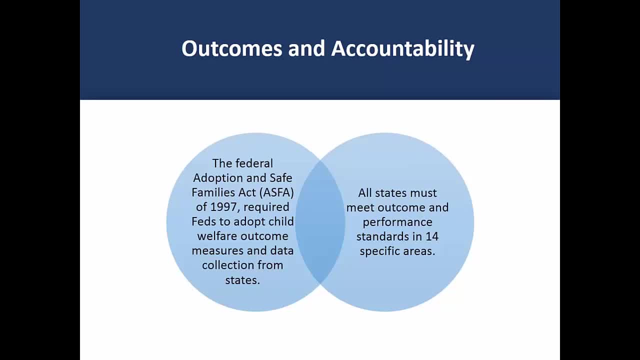 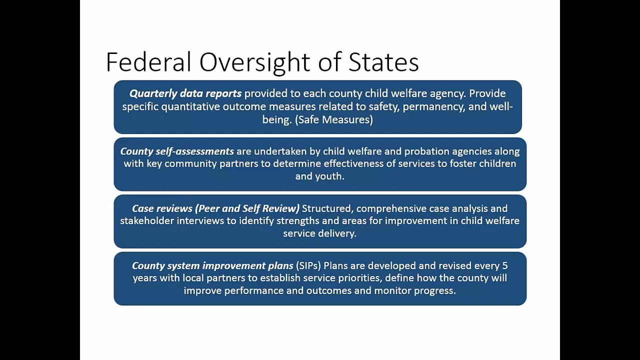 monthly performance matrices. Each part of this plan is what's driven a 40% reduction in the number of foster youth and out-of-state placements since 2000.. Next slide, please. There are four processes that federal authorities use requiring states to implement this oversight. 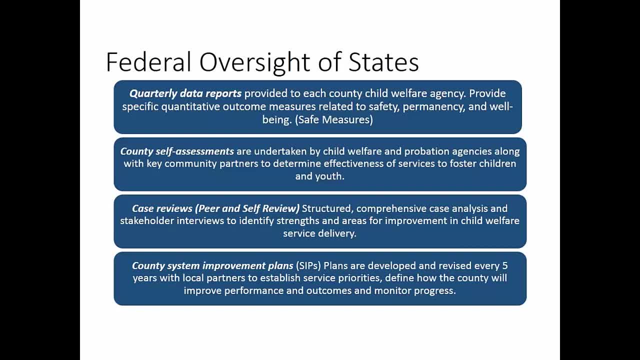 effort. Each county or jurisdiction must conduct quarterly data reports. Each county must conduct a self-assessment process along with its probation partners. Each jurisdiction is also responsible now for conducting case reviews that involve a structured analysis of the documentation of care provided within a child welfare services. 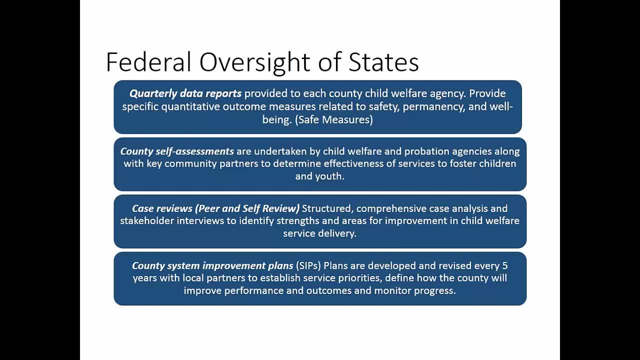 care episode. These three elements roll up into a five-year planning, which is commonly referred to as a system improvement plan. These plans are monitored by the county, of course first, and then by the state, and ultimately make their way into a federal report. 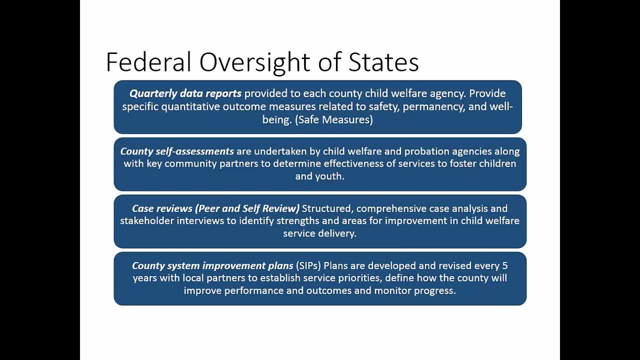 So, Richard, do counties report this data directly to the federal government for these types of outcomes? Well, typically the state would aggregate all the county and federal reports. So, Richard, do counties report this data directly to the federal government for these types? 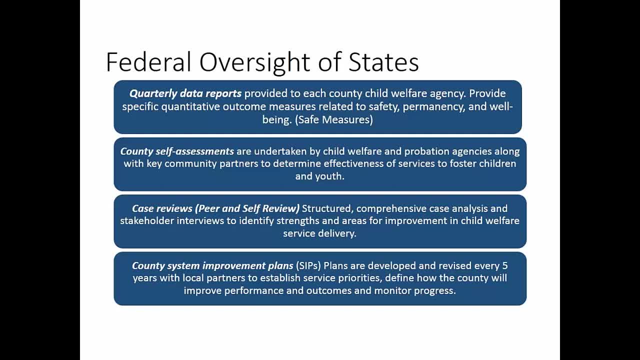 of outcomes. Yes, So the state would collect all the county information and then would make a statewide report to the federal authorities. Only in the cases of specific grants awarded to a county would there be an independent reporting from the county directly to the feds. 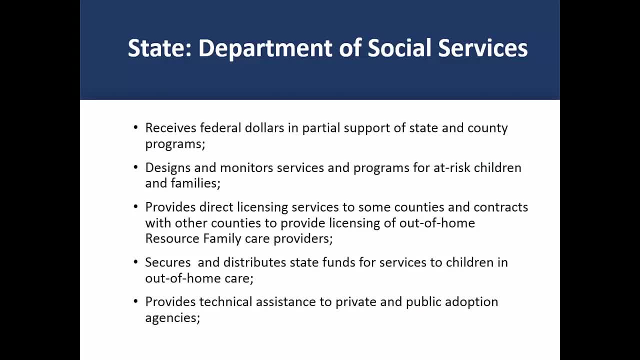 So let's take a look at the state-level services. California is one of about a dozen states that uses a state-administered, county-implemented model. Other states have a state-administered and state-office-delivered system with no county. 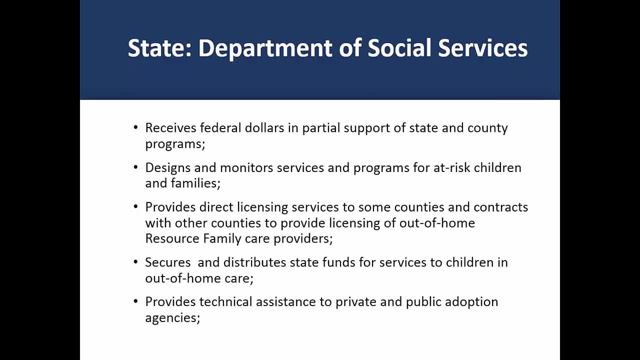 specific jurisdictions. Each of California's 58 counties conducts its own child welfare services, while CDSS, the state agency serving as a large administrative services organization, monitors and supports counties through regulatory oversight, administration and the development of program policies and regulations. 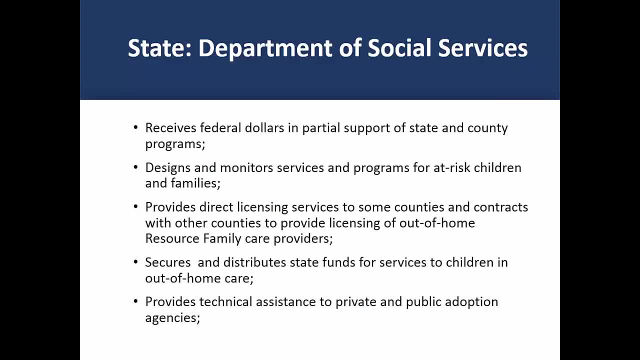 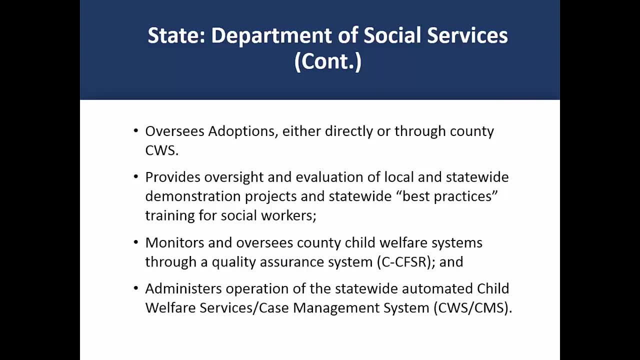 Within that large state department, two divisions are most critical to youth and families, those being the Child and Family Services Division and Community Care Licensing. Okay, Now let's take a look at the State-Administered Services System. Among many duties, CDSS oversees most aspects of the county-delivered service model. 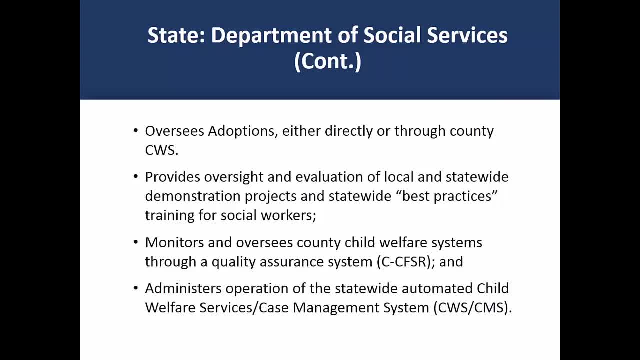 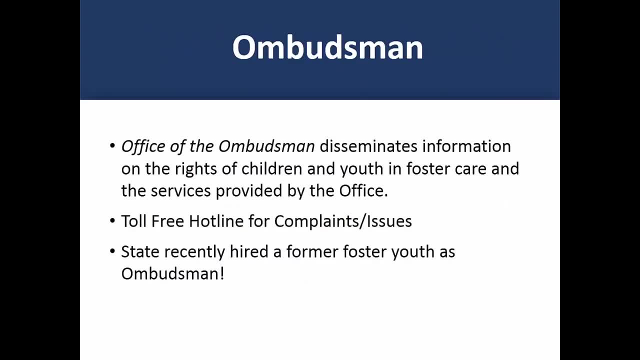 Those administrative and regulatory processes include training, best practice implementation, quality assurance and the statewide data system known as CWS, CMS. The Department of Social Services also has an independent office of ombudsperson, which investigates and attempts to resolve problems. 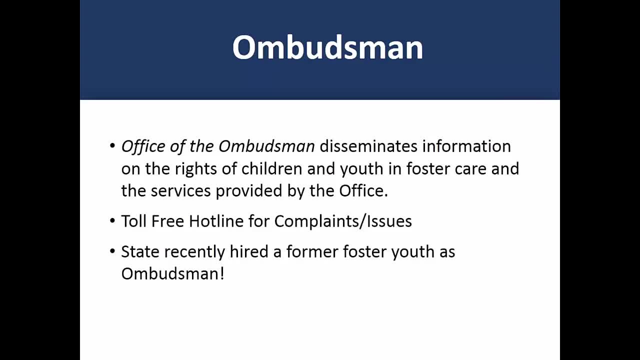 complaints made by or on behalf of children placed in foster care and compiles all complaints received in an annual report to the legislature. All county child welfare workers are required to provide foster children with information about the Ombudsman's office. Counties also have a local ombudsperson. 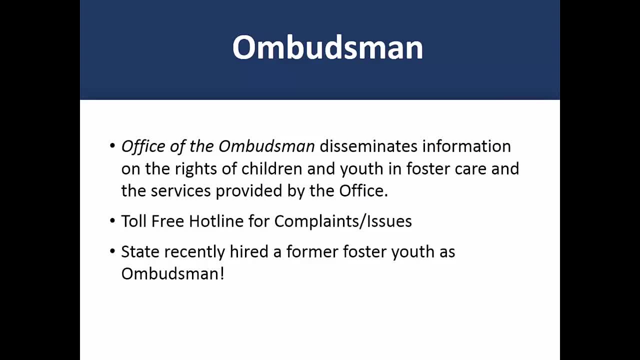 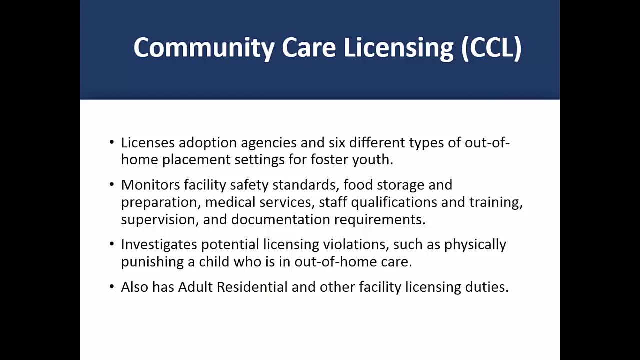 The state has recently championed innovative youth representation by employing a senior manager ombudsperson who has lived experience in the foster care system. This may be a first-in-the-nation effort on California's part. One of the department's major objectives is to assure that all of the 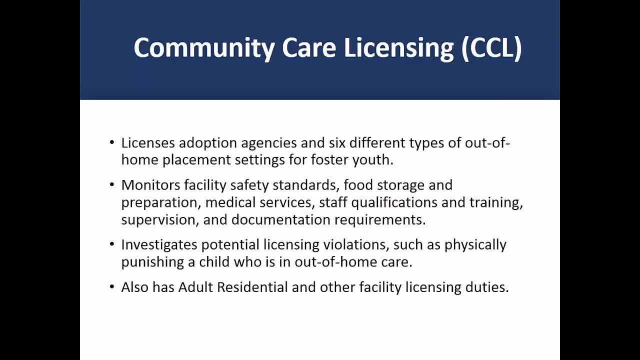 various community-based agencies that serve foster youth are safe and offer a high quality of service. This licensing process oversees a host of different types of service: out-of-care, out-of-home services, including foster family homes, small family homes, foster family agencies, group homes and. 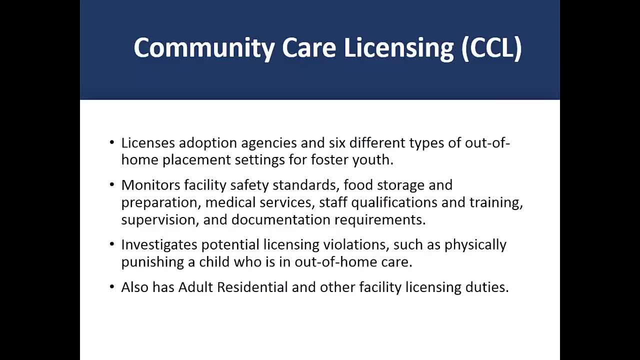 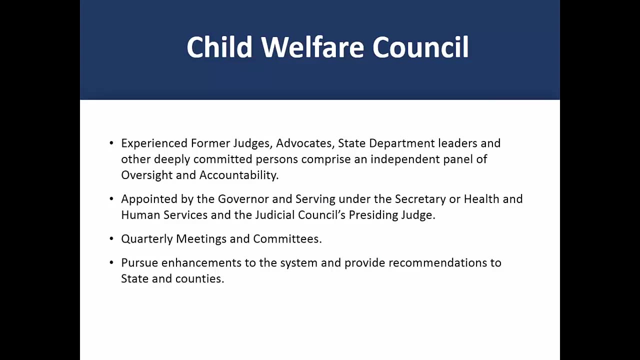 community treatment facilities and transitional housing placement facilities. They each have their own set of licensing expectations. CCL will also oversee licensing of the new short-term residential treatment programs. Separate but related to the State Department is the Child Welfare Council. A number of years ago, California identified a desire to bring together diverse leaders to 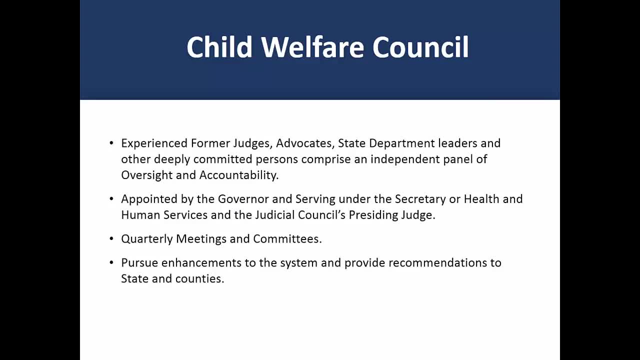 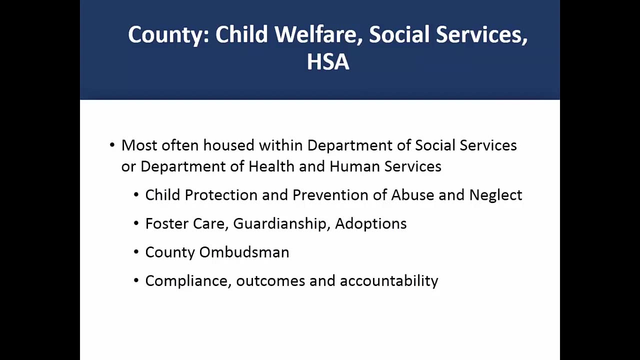 provide independent advice to CDSS and its partners. The Child Welfare Council was born and today meets quarterly in a vibrant, day-long conversation in pursuit of enhancements to the welfare and related systems. Now let's take a look at the county level agencies Under guidance and. 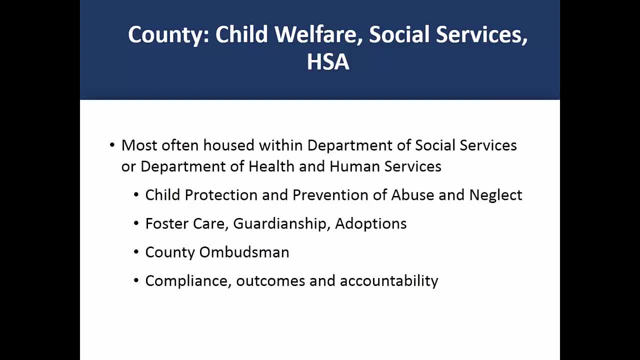 oversight from CDSS. each county delivers its own CPS and welfare related services. These can generally be broken into four kind of functional areas, including child protection for the prevention of abuse and neglect, foster care, guardianship, adoptions and permanent planning a. 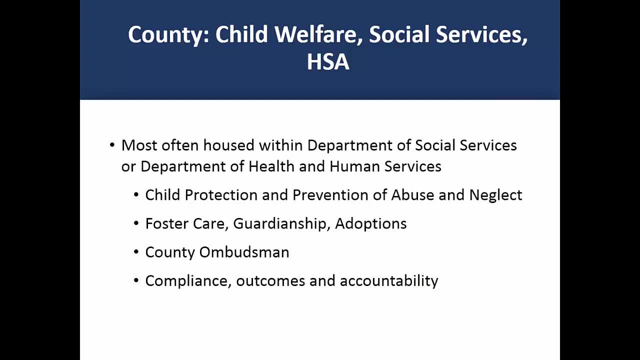 county ombudsman's function, which we just talked about, and compliance outcomes and accountability. So, Richard, can you tell us a little bit more about the relationship between the county ombudsman and the local Child Welfare Authority? Sure, it's an interesting relationship. 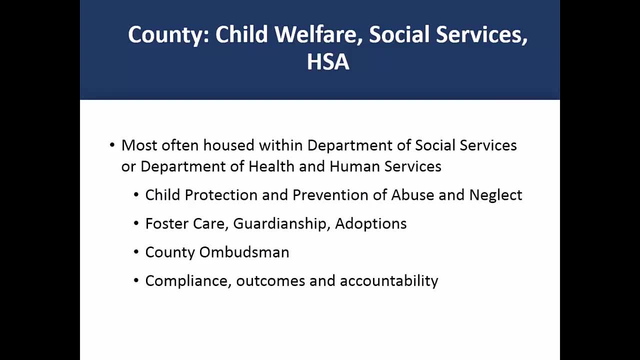 While the ombudsman's office and function is hired by or provided by the local Child Welfare Services Authority, its role and intent is to provide an impartial and objective ear for consumers who have concerns about the the agency's work. It reports to the county but liaisons to the state. 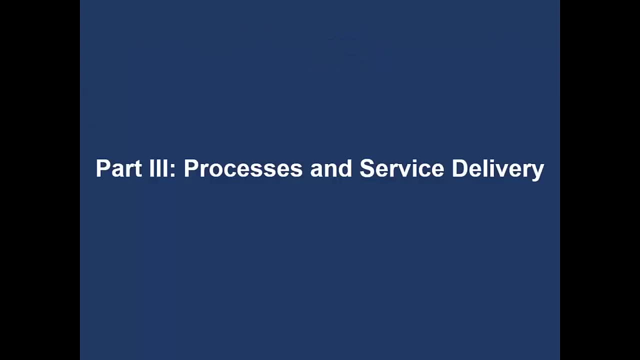 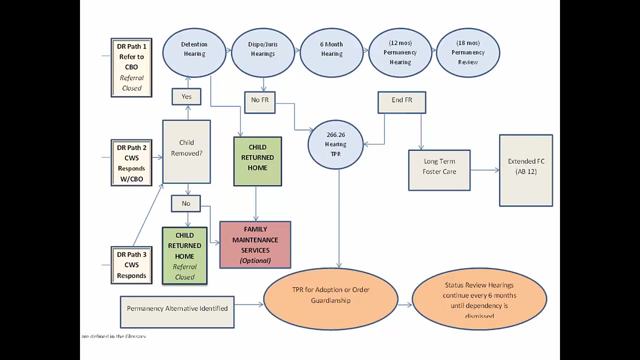 ombudsman's office as independently as possible. Now that you understand the structures of the federal, state and county authorities involved, let's take let's take a look about at what the actual services look like. Each county has a 24-hour telephonic triage service. This busy schematic outlines the major 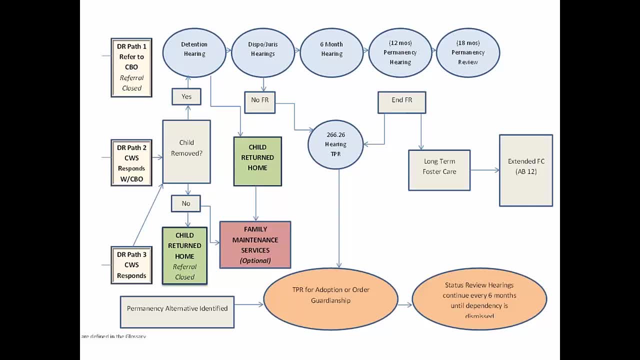 services and steps along the journey of a family in the child welfare system. The Child Welfare Services Authority's actions are typically represented here in the tan or taupe color. The court's role is structured in the blue-hued circles along the top. There may be, of course, 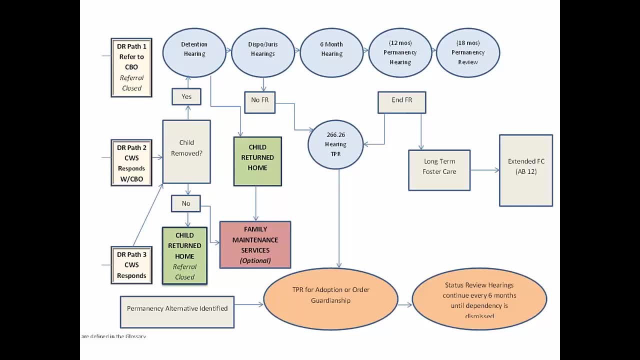 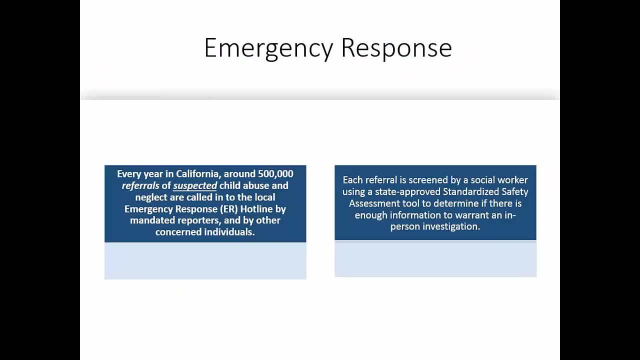 local rules or agreements that adjust in minor ways in this general process. The slides that follow, of course, will explain much of this process in greater detail. Each county has its own telephone number for reporting suspected abuse. This part of the CWS response is known most often as emergency response or ER. 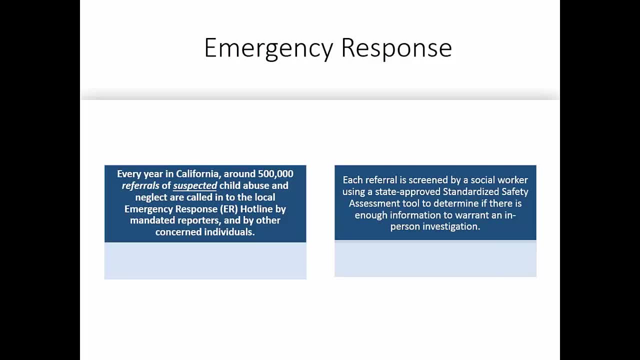 services. The standard safety assessment system evaluates the safety, risk and needs of children and families who are referred to the Child Welfare Authority. Most counties have senior or supervisory staff that review all decisions. Unlike decades ago, tools are in use today which most often inform the investigation and conduct of 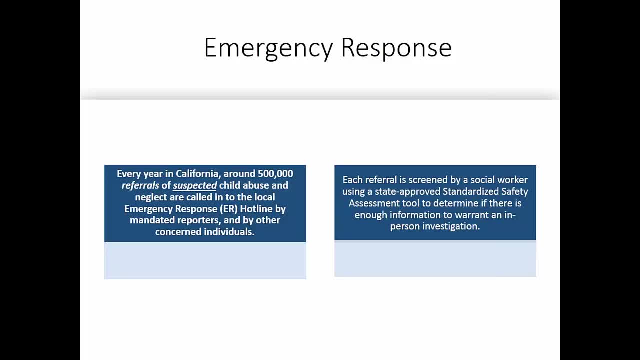 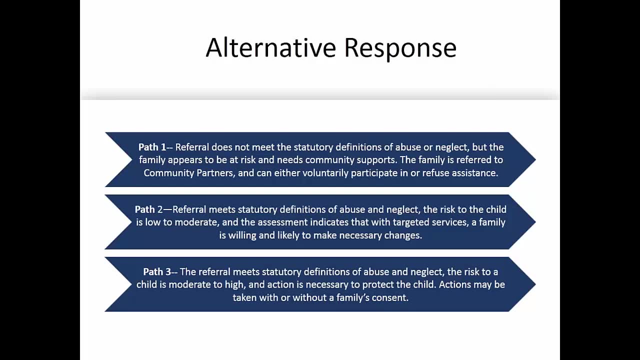 the investigation on behalf of children and families in order to protect parental rights and assure due process. Differential response was pioneered in the 1990s in Minnesota and has been in use in California for about 15 years. Depending on circumstances, a traditional investigation by a child welfare agency is not needed in every case or every. 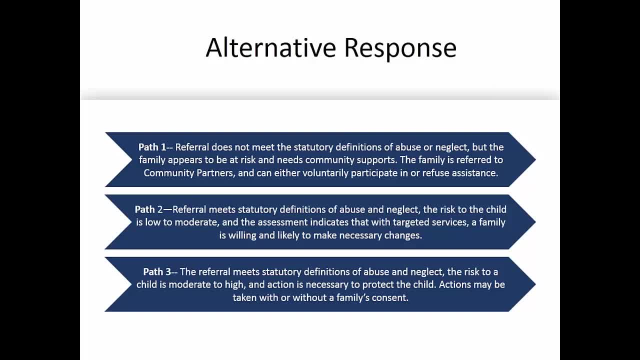 referral, While maintaining a fundamental commitment to child safety. differential response is a strategic three-path approach that's in use in about 40 California counties. Path 1 represents those cases which have minimal risk, usually resulting only in a referral for supports or services. 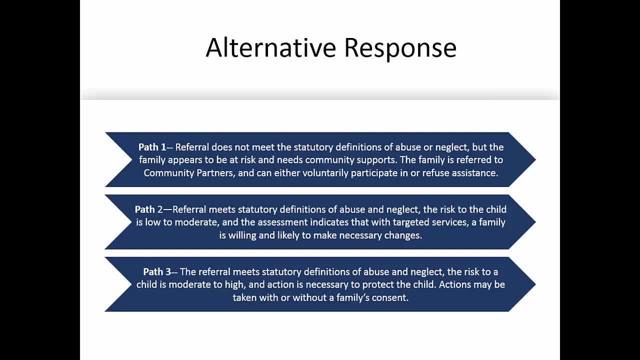 Path 2 focuses on voluntary involvement in services. However, in the interest of protecting the child, the authority of the court may be utilized. Path 3 is most similar to the child welfare system's traditional response, in which case efforts are made to engage the family, especially non-offending parents or 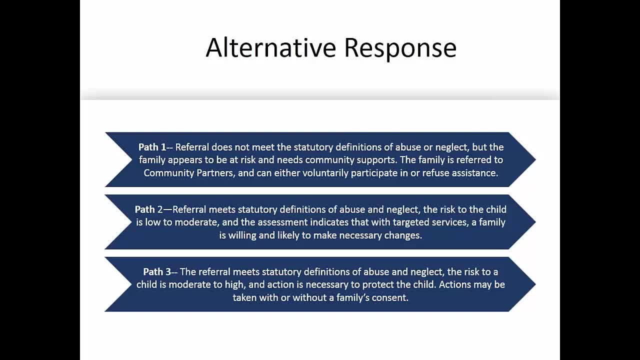 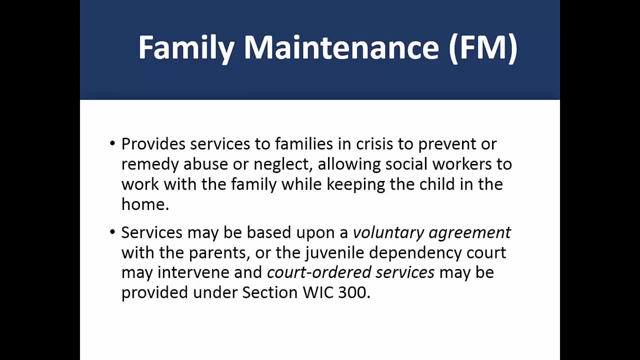 other protective adults to preserve the connections between the child and other family members. Ideally, bio caregivers are willing to engage in assuring their children are safe and well. Family maintenance cases typically allow families to be together without detainment. The family maintenance funds that counties receive. 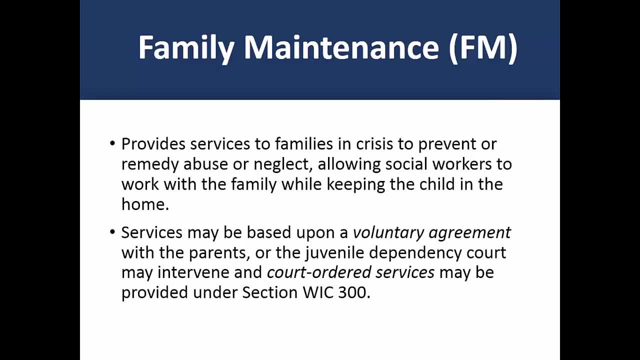 from the state are typically available for up to 12 months of service. Court ordered family maintenance services may be extended by six-month intervals and continued indefinitely if it can be shown to the court that the objectives of the service plan can be achieved within the extended time period. 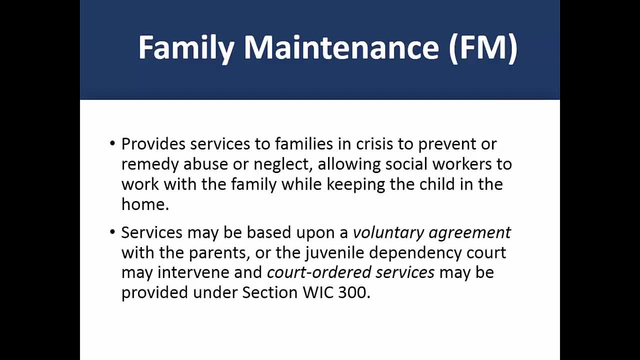 And if the services can be provided within the county's child welfare services allocation. Family maintenance services are provided based on a case plan developed by a child welfare worker and the family, And they include, but are not limited to, counseling, emergency, foster care, respite care, emergency and. 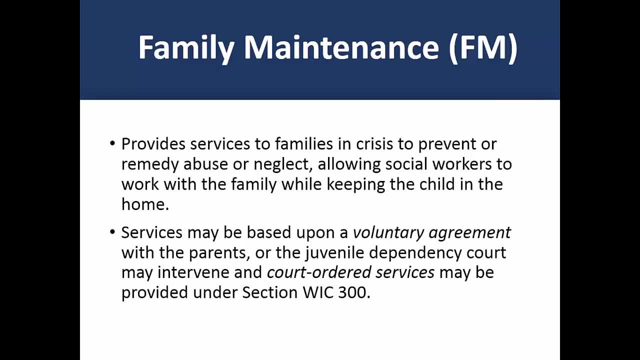 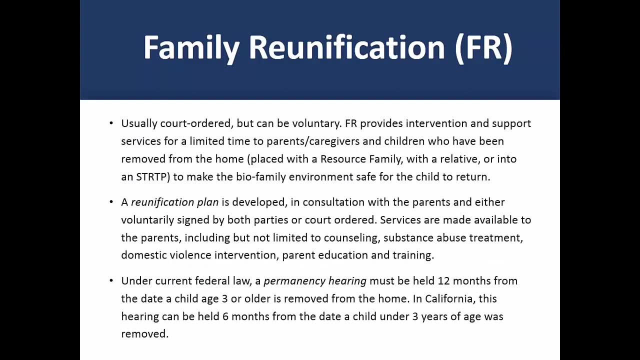 home caretakers, substance abuse treatment, domestic violence intervention and services, parenting, education and others. Family maintenance ensures that counties have ability to protect the minor while working with families to minimize disruption and trauma In cases where a minor has been removed. counties 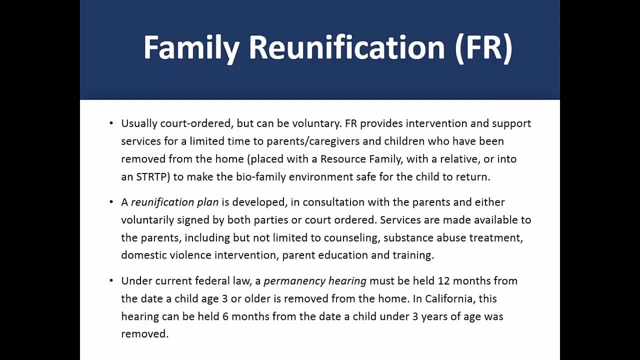 seek diligently to reunify the family as quickly as possible. Family reunification services may be extended beyond six months for a child under the age of three, or beyond 12 months for a child over the age of three, as long as the court finds that there is substantial probability that the child will be returned to the physical. 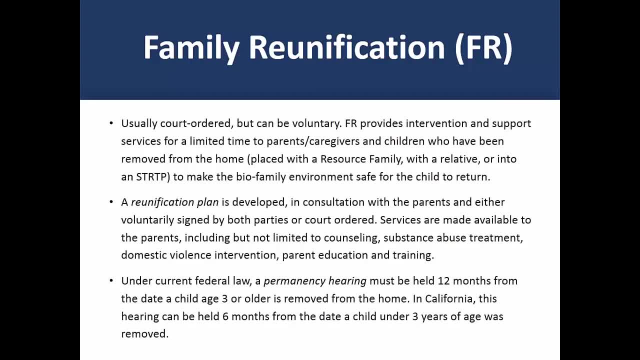 custody of his or her parent or guardian within the extended time period or that reasonable services have not been provided to the parent or guardian. Child welfare agencies are required to file a petition to terminate parental rights when a child has been in foster care for 15 of the past 22 months. The service plan must be satisfactorily fulfilled for. 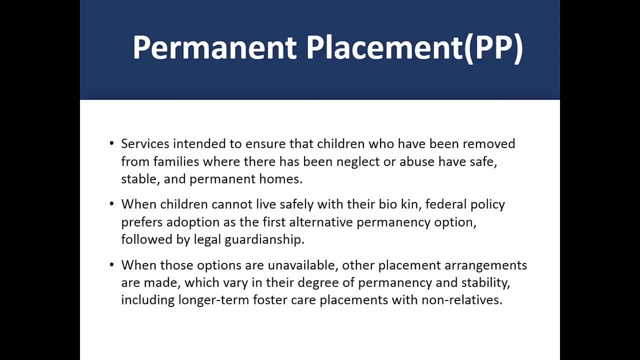 the child to be returned home. In cases where longer-term out-of-home care is necessary, permanent placement services apply. There are many forms of permanency. Permanent planning services begin concurrently to other services and are intended to assure safe and stable care for minors placed away from their primary caregivers. Adoption is the preferred long-term 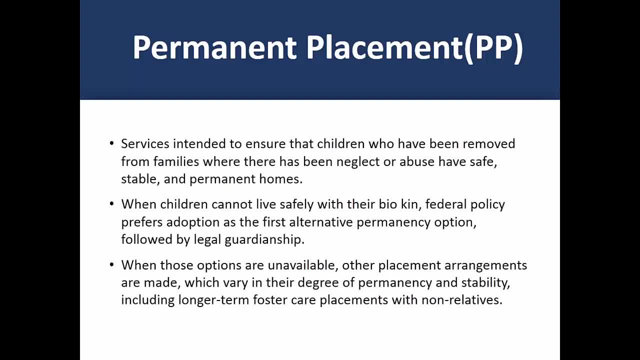 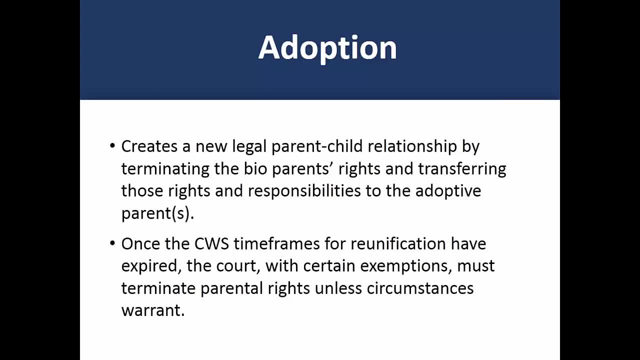 placement option. of course, We'll talk more about adoption shortly. When intact families cannot be successfully served, they are not eligible for the child's care. The child's care must be fully served. Adoption is often preferred as the second plan To prevent. 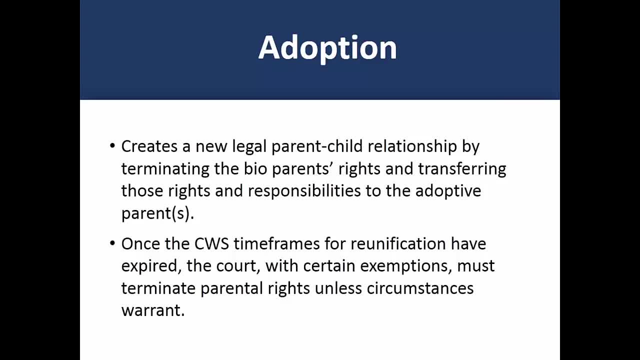 completely severing a child's existing family connections. California adoption law now allows parents or relatives to enter into a post-adoption contact agreement with the adoptive parent, subject, of course, to court approval, where parents or relatives continue receiving information about and or maintaining contact with the child. Examples of exemptions include a child 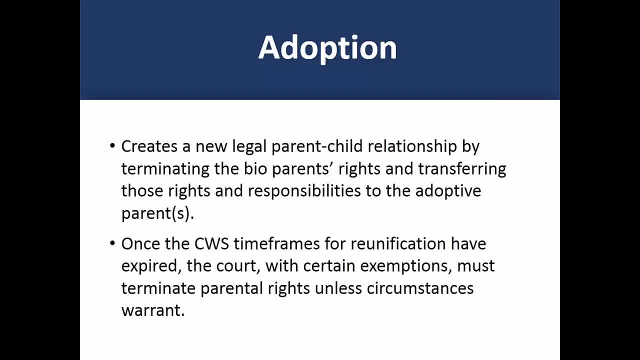 whose parents have maintained regular contact, where the child might benefit from continuing the relationship with the child, or a child whose parents have maintained regular contact, where the child has been in a relationship with the child, a child who is 12 years of age or older and objects to being adopted, and if the adoption will interfere with the 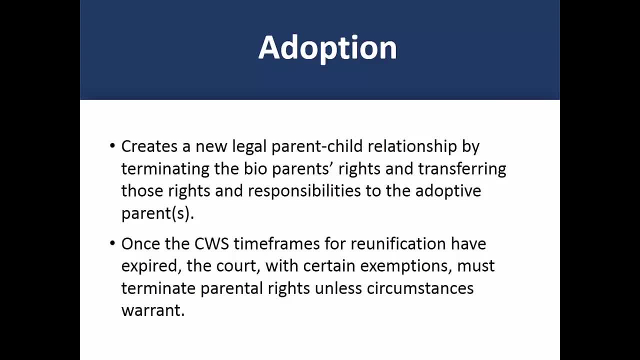 connection of a Native American child to his or her tribal community or the child's tribal membership rights. In some Native American tribes, adoption with termination of parental rights can mean the child loses citizenship in the tribe along with the benefits received from tribal membership. so these can be sensitive issues. Timeliness to adoption is a major 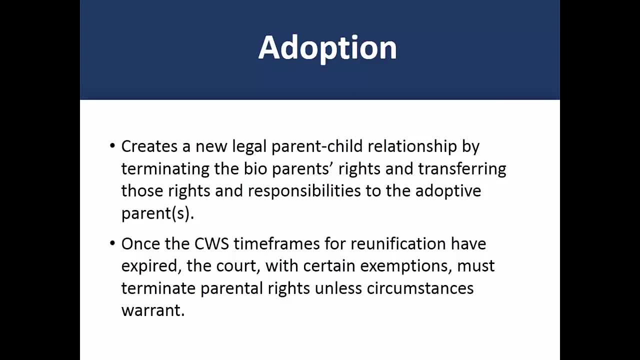 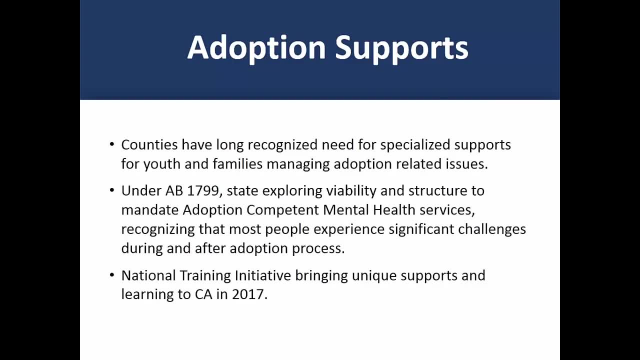 statewide improvement in the last decade and contributes to stability and well-being for more often than not. Aid to adoptive parents funding supports youth in and after adoptions. Historically these would include counseling, case management or community supports. California partners are excited and of particular interest to mental health partners and providers in that. 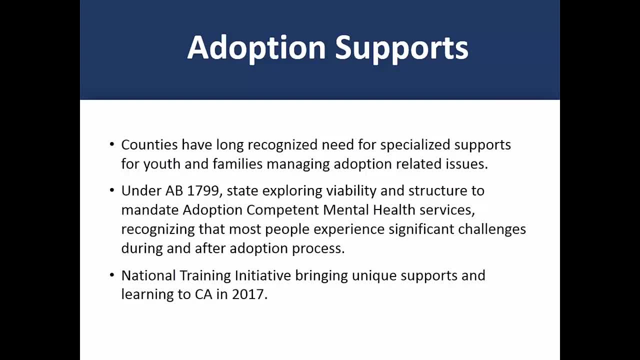 the state has been identified as one of eight national piloting sites for the development of adoption-competent clinicians. We are recognizing the need for specialty mental health intervention throughout and following the adoption process. Nearly 2,500 California practitioners have been signed up and will be trained by the end of 2018.. 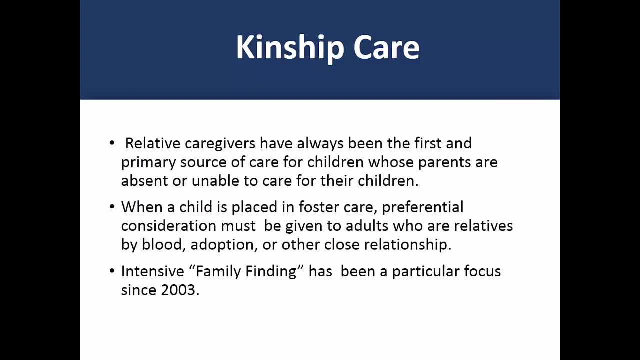 Being in foster care can be very stigmatizing. One way this can be greatly mitigated is by having caring extended family members provide care and supervision to the victim. California youth in dependency are placed into kinship settings in a program that is designed to 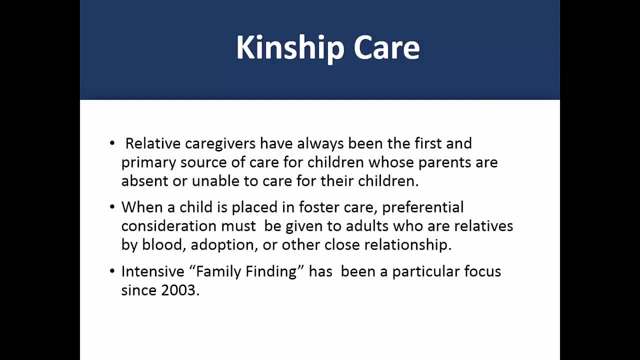 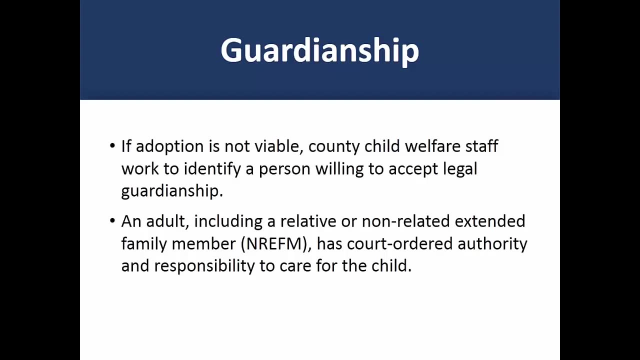 provide care and supervision to the child's biological family. This is a significant improvement since 1998, due largely to timely location and connection making with extended family members. We call this family finding Similar to adoption, although guardianship does not provide the same level of permanency. 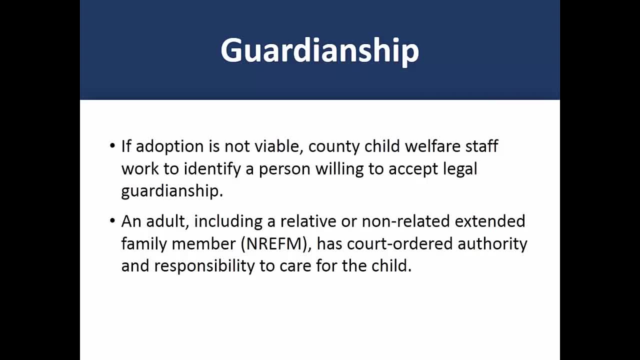 that is afforded through adoption. guardianship can facilitate continuity of formal and legal ties to the child's biological family, Which may be the case if the child's biological family does not provide the same level of support. The child's biological family may be in the child's best interest. 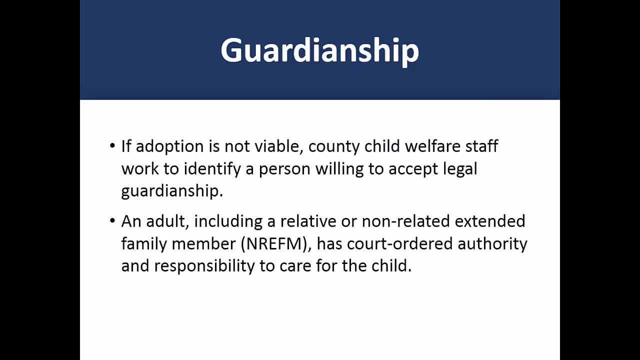 Legal guardians have authority to make decisions on behalf of the child that a biological parent would make, but have no legal obligation to support the child financially. The biological parents continue to be legally required to provide financial support for the minor. If a relative becomes a guardian, the child welfare and dependency court cases may be. 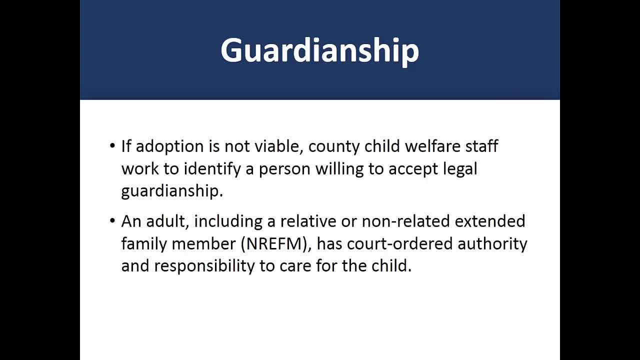 closed. Through the Kinship Guardian Assistance Program, known as KINGAP, the relative may receive ongoing financial assistance for the child in the same amount that the child would have received if he or she had been in a foster home. Most non-related legal guardians. 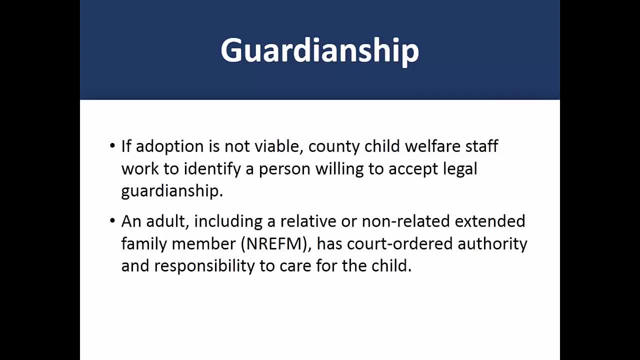 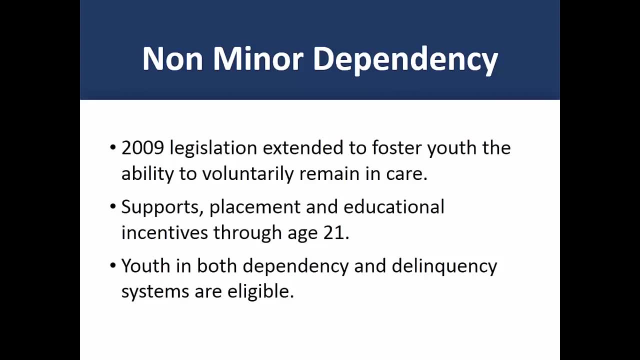 receive similar financial assistance under the state AFDC foster care program and remain under the supervision of the court. Joining many other states, based on widely celebrated national research from the University of Chicago, California now makes foster care status and its supports available to youth. 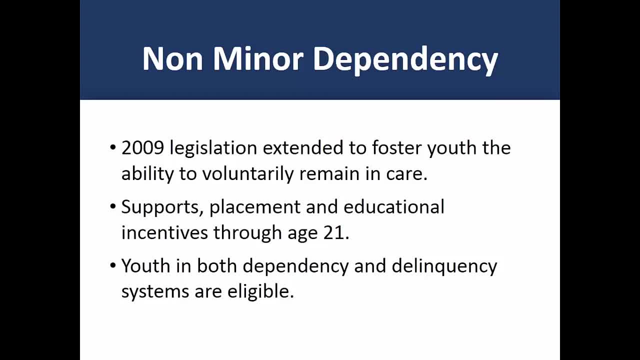 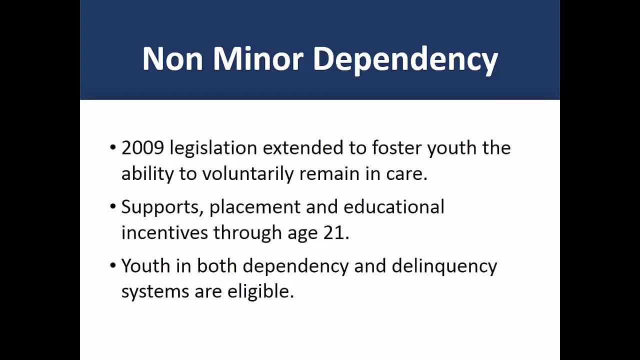 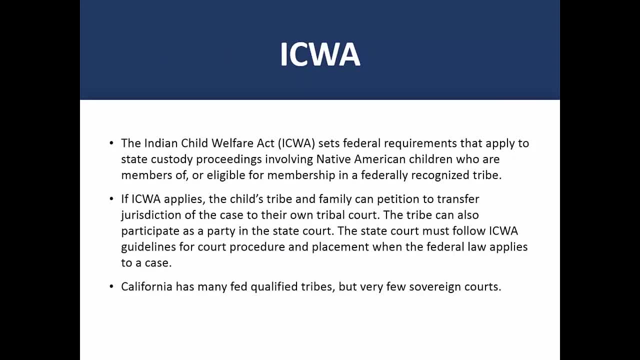 declining arrest rate in the last seven years. Let's spend a minute talking about the Indian Child Welfare Act. Tribal partners are critical to successful foster care for youth with native identity. ICWA, the Indian Child Welfare Act, provides unique supports and is intended to ensure. 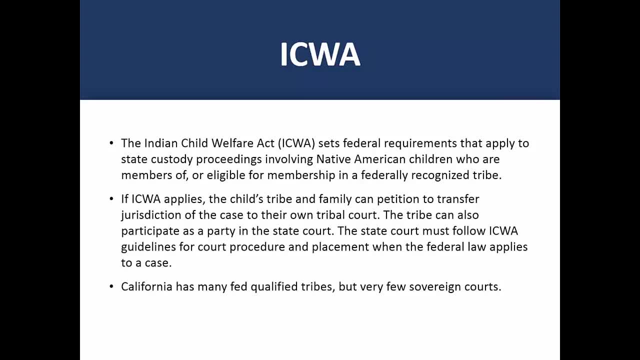 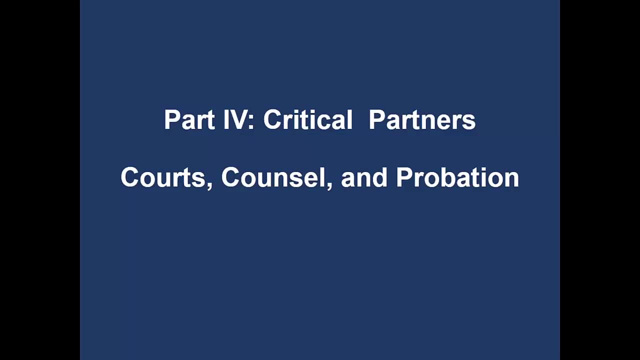 native youth are served in a fully culturally proficient way manner. Child Welfare Service's, county partners and tribes work together to assure cultural and ethnic supports are accessible and available to the youth and family. While California has many tribes, there are very few tribal courts. 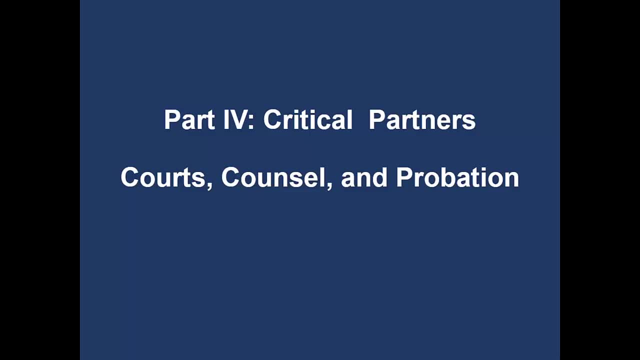 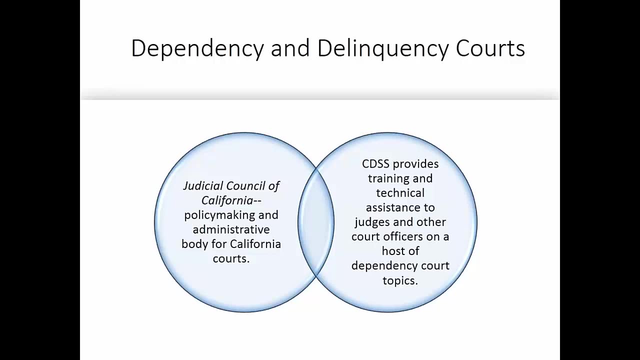 Let's talk now about some of the Child Welfare's Outstanding Partners. Independency: Formerly known as the Administrative Office of the Courts, the State Judicial Council is the statewide administrator of county court services, Under the leadership of the Chief Justice and in accordance with the 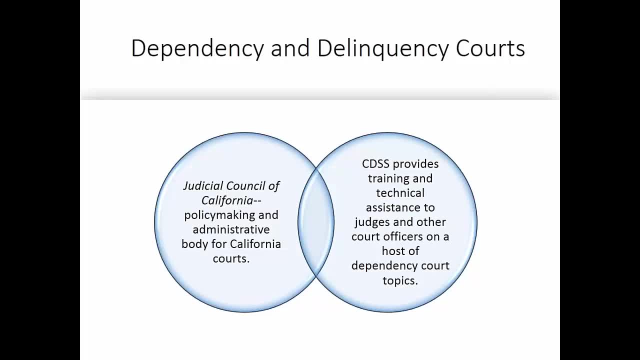 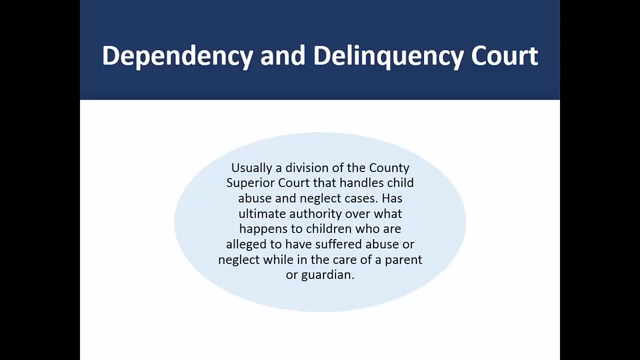 California Constitution, the courts deliver guidelines to themselves and to make recommendations annually to the governor and legislature, and they also adopt and revise California's rules of court in the areas of court administration, procurement, practice and procedure. The Welfare and Institutions Code- section 300,- provides. 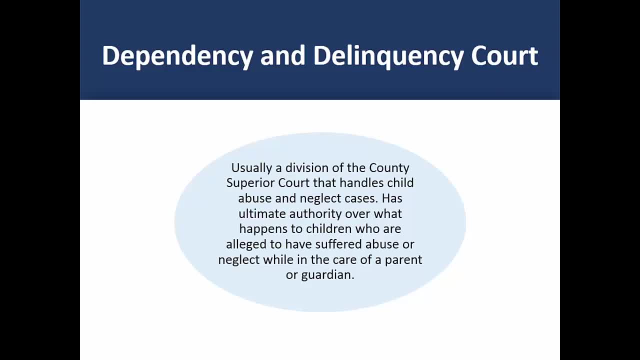 the legal basis for juvenile court jurisdiction and authorizes the court to remove children from the care and custody of their parents if such action is necessary to keep the child safe. Large counties may have two or three juvenile officers, while medium and small counties may have a single judge or 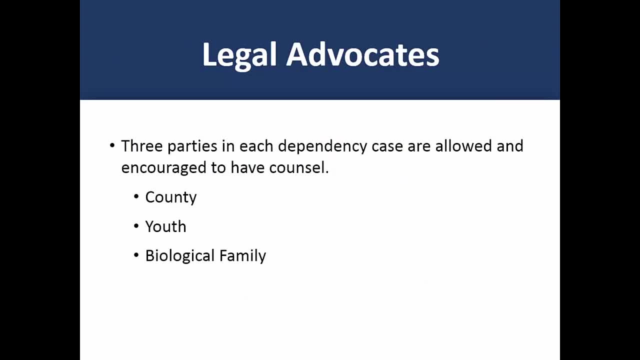 commissioner, who may have other duties. There are other legal advocates that partner with courts and child welfare authorities. The state constitution provides that all parties to a CWS proceeding have legal advice. County departments have an attorney assigned. the court assigns a lawyer for the youth and family members who may also bring. 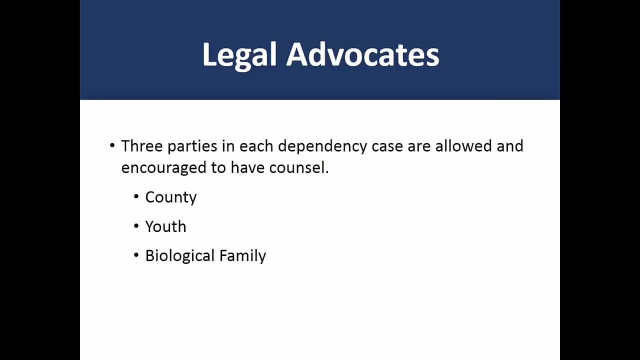 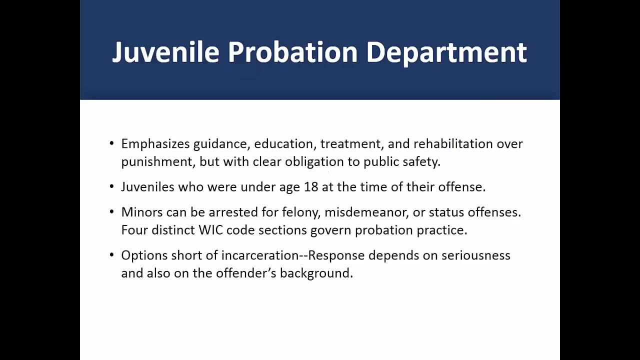 their own counsel or have one appointed at taxpayer cost. In most counties, these advocates work collaboratively to help the youth and family navigate the system and control the system and quickly reunify without additional trauma. Occasionally, dependency cases can become adversarial. One key partner working with child welfare is the. 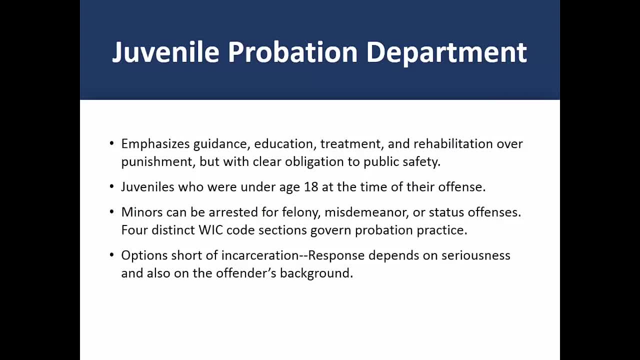 juvenile probation department. In addition to local law enforcement, county probation departments and juvenile courts work with local school districts and child welfare and behavioral health departments. County probation departments are also responsible for operating juvenile halls, camps and ranches. At the state level, the Division of Juvenile Justice maintains: 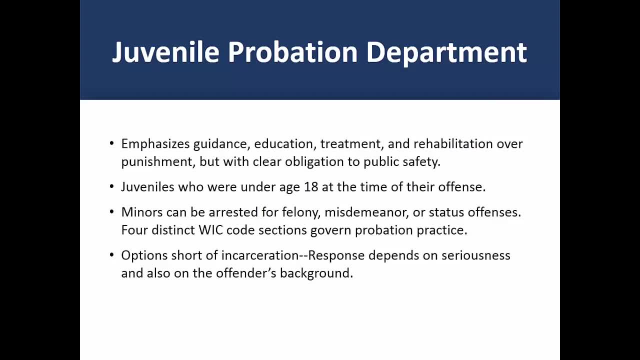 three secure facilities and a conservation camp for lower risk offenders. For example, a 15-year-old arrested for the first time for skipping school might be counseled and released. At the other extreme, the most serious cases may be directly filed on or remanded to the adult criminal system. 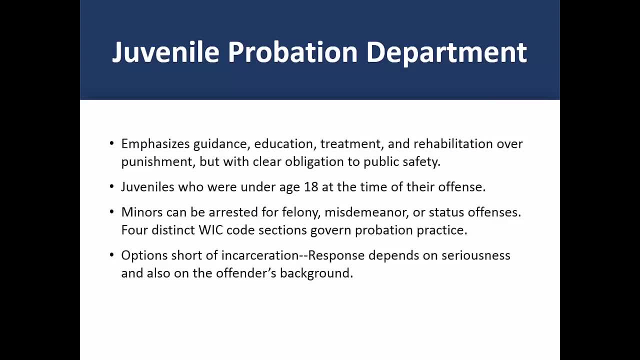 Most of the time, however, law enforcement refers the arrestee to a county juvenile probation department. About half the time, the probation department either closes the case or prescribes informal probation or a diversion program, which might include education, community service or restorative justice types of services. More serious cases: 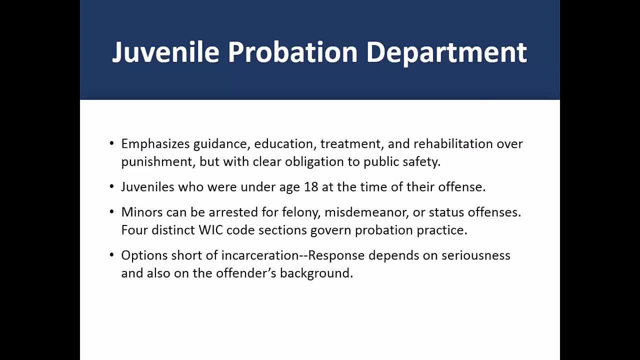 warrant a juvenile court hearing, but judges have a range of options short of committing youth to a county facility. Of the approximately 150,000 juvenile arrests made in 2011,, for instance, only 11% resulted in confinement and fewer than 1% resulted in commitment to a Department of Juvenile Justice facility. 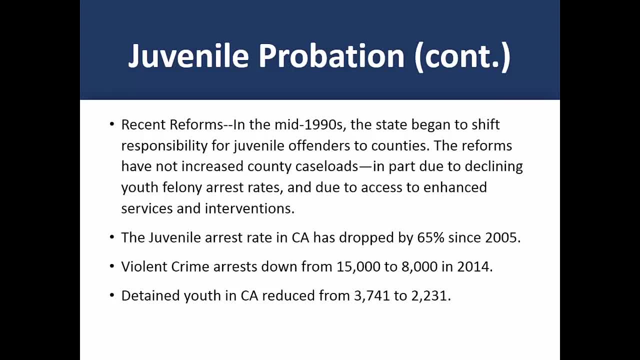 A 2007 reform permitted counties to commit only the most serious offenders to state facilities. Between 2007 and 2013,, the year-end number of juvenile offenders in the Department of Juvenile Justice institutions and camps fell from just over 2,100 to under 700.. The share of youth in these DJJ facilities for 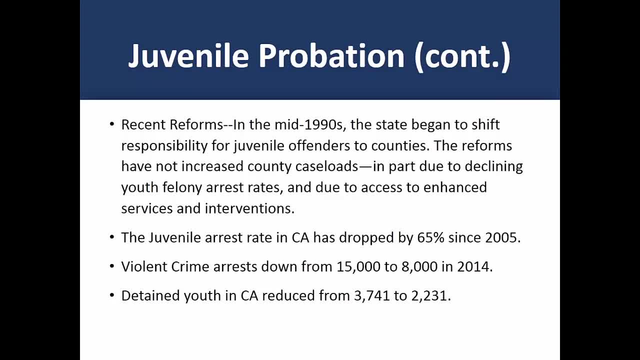 homicide increased from 5 to 12.4 percent and for assault from 32.2 percent to nearly 40 percent. A subsequent reform gave counties responsibility for all offenders released from DJJ, resulting in a drop in state parole numbers from 2,462 to 0 between 2007 and 2013.. 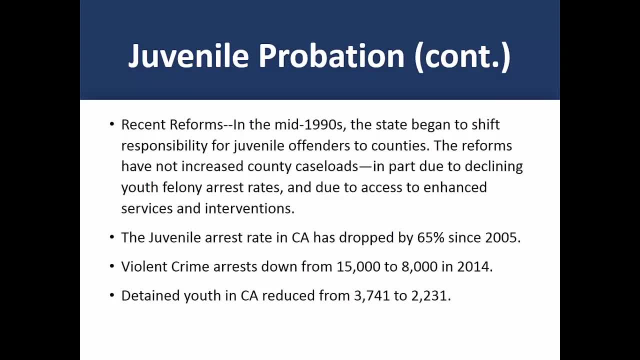 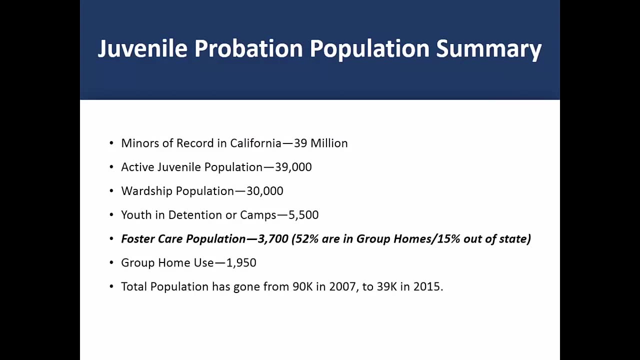 One contributing factor is that between 2007 and 2012,, the juvenile arrest rate fell by 42 percent to its lowest level in decades. This trend mirrored a general decline in felony arrest rates for young adults across the state. Here's a quick look at some big picture probation demographics: There are 27 juvenile detention. 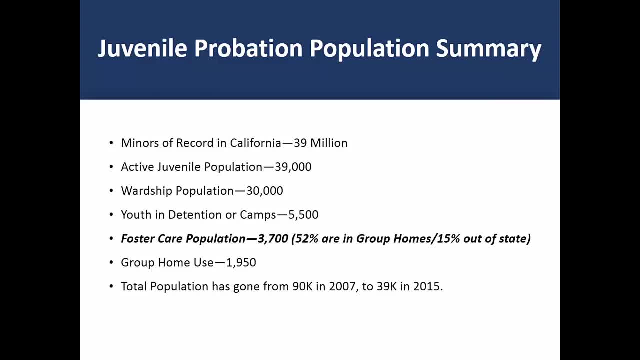 facilities and about 55 camps run by county agencies. Of the nearly 40,000 youth with open cases in the probation system, about 80 percent are 602 misdemeanor offenses that receive services that typically involve community supervision, Rates of foster care and group home care for youth. 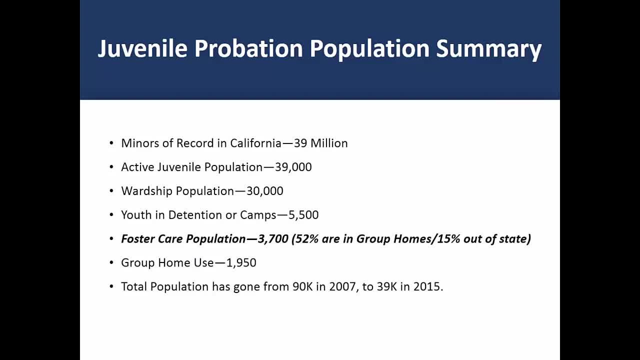 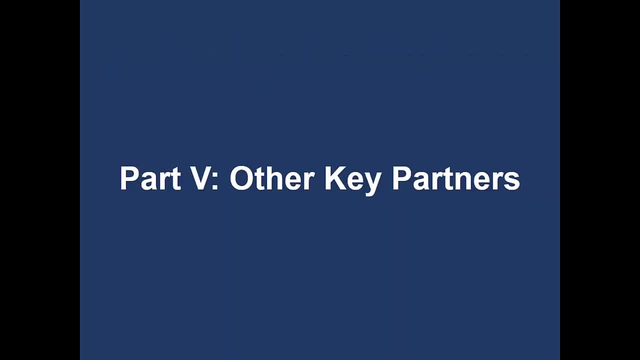 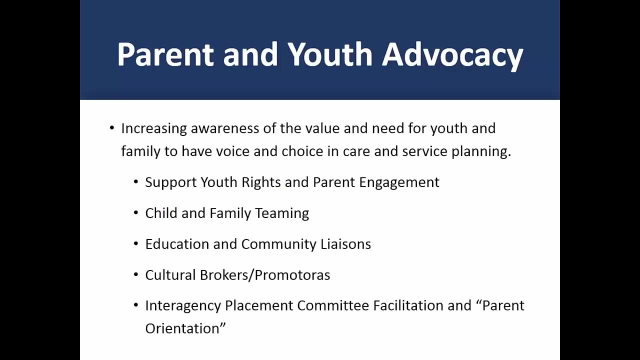 involved in the delinquency system have declined by more than 50 percent, which reflects outstanding work on the part of the county probation departments around the state. Welfare agencies have other critical allies helping in their work. A growing body of research has shown that family and youth both do better when someone with lived experience can walk. 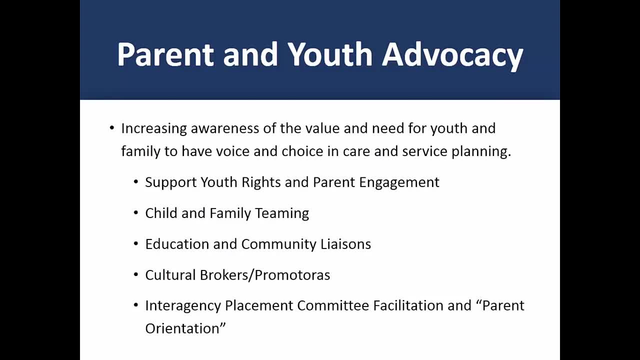 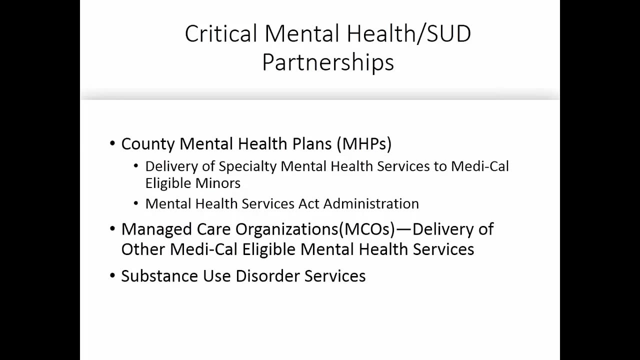 with them through the system, helping to navigate and support them. These bullets show some the roles played by youth and parent partners. These partnerships are either purchased by the agency via a contract or, in some cases, may be employed directly by the county department. Increasingly, there is awareness that foster youth most often need. 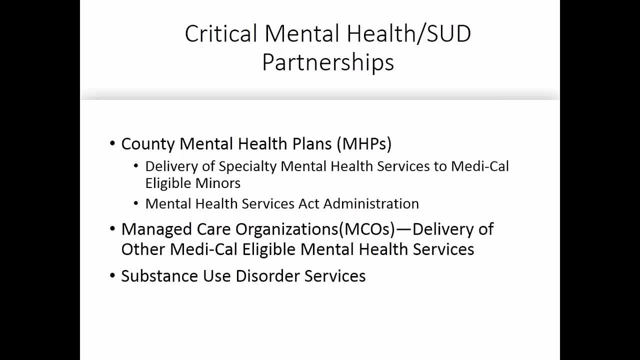 intervention or support from the mental health community to effectively cope with their trauma. All foster youth are automatically eligible for Medi-Cal and, under recent KDA settlement agreements and the continuum of care reform, all youth are screened for mental health needs and many are assessed and found to. 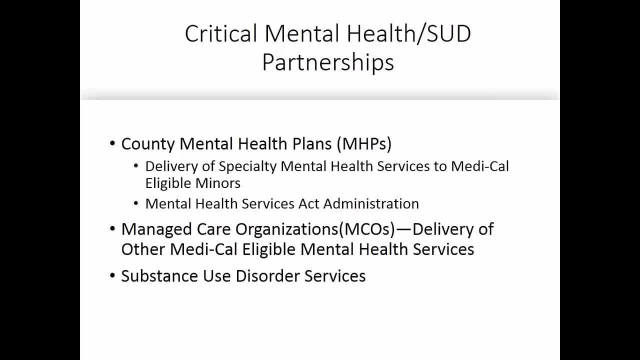 meet medical necessity criteria to receive mental health or behavioral health care. Since 2014, county mental health plans have been invited to coordinate with regional or local managed care companies who were awarded contracts to deliver care to less acute beneficiaries. Counties and managed care organizations have agreements in place which are intended to assure a timely 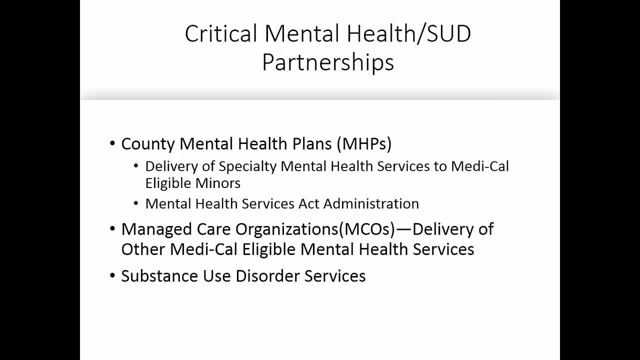 assessment and referral and care coordination for all Medi-Cal eligible youth, including foster youth. Substance abuse services are historically not well-funded at the federal or state level, especially for youth. There are limited funds available and most counties have some SUD services available, usually accessible through the mental health plan. So Richard is Medi-Cal. 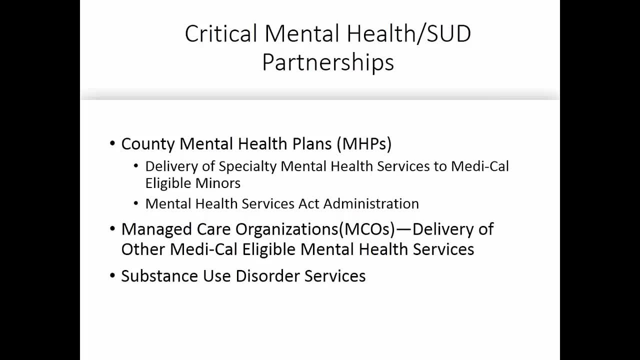 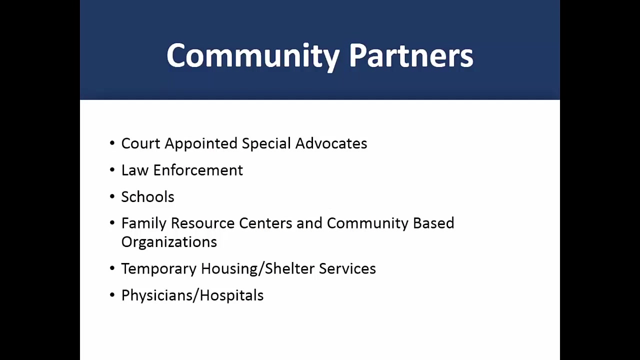 eligibility: the same for former foster youth as those currently in the system. The eligibility criteria are the same same, Kim. While there are special services available for former foster youth through the legislation commonly known as AB 12 or non-minor dependent services, the eligibility criteria themselves are the same. Other partners: 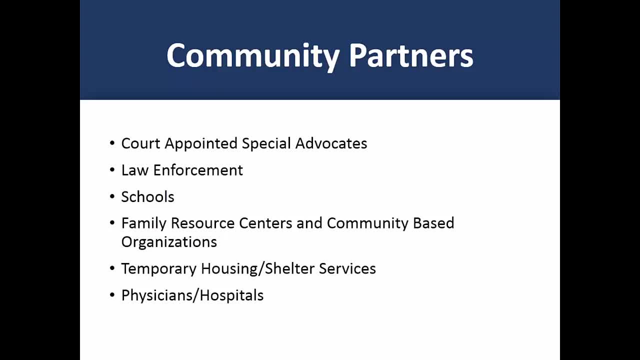 include those listed here. Each of these entities provides a mandated and often valuable adjunctive role to the protection and safekeeping of a minor. The scope and reach of these services will vary by county, but often mental health clinicians working with Child Protective Service involved youth will. 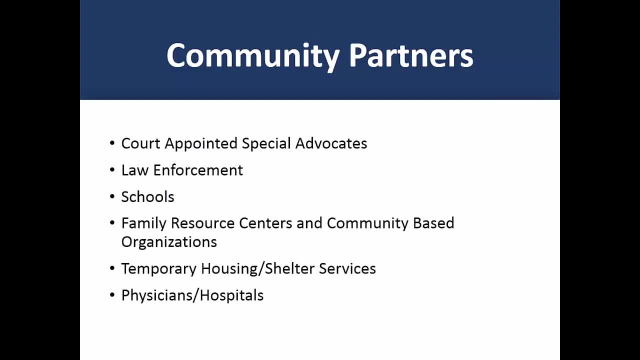 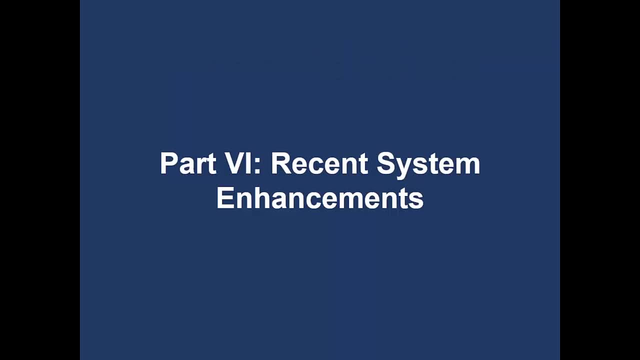 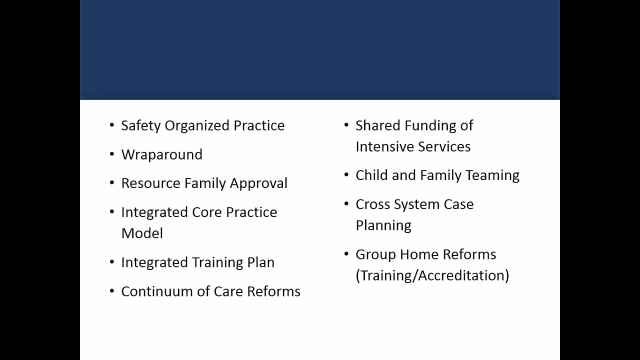 want to be aware of the partnerships and resources available in the parallel health and social service systems represented in this slide. Let's talk for a moment about the last 15 years of improvements that have been implemented and our research. Since 1997, counties and state agencies have developed and implemented many 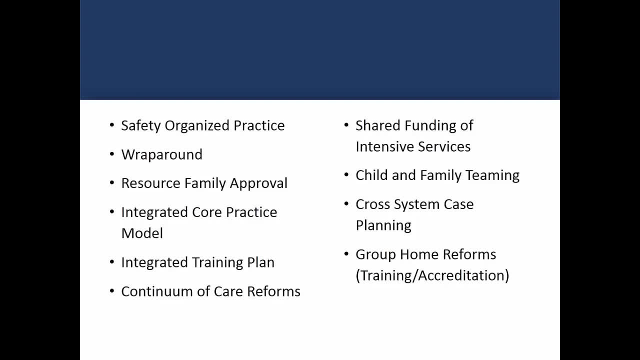 evidence-informed or evidence-based improvements, Safety, organized practice, wraparound, child and family teaming and others all share a major objective of assuring authentic engagement with biological family members and service planning that seeks to connect the youth and family to their natural support. 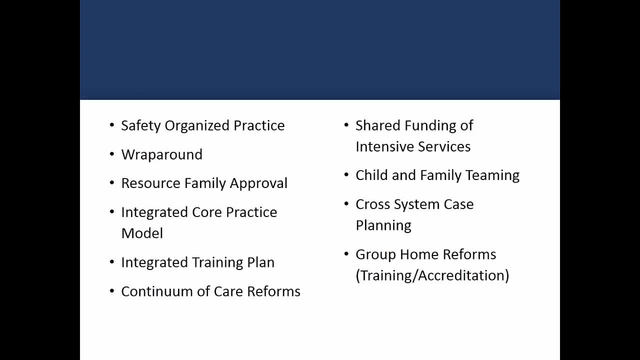 Where they can be most effectively served and where stigma is minimized. Resource: family approval enhancements are intended to assure any caregiver is fully trained and supported. Soon the state will have an integrated core practice model which will be a cross system guide which captures how staff in 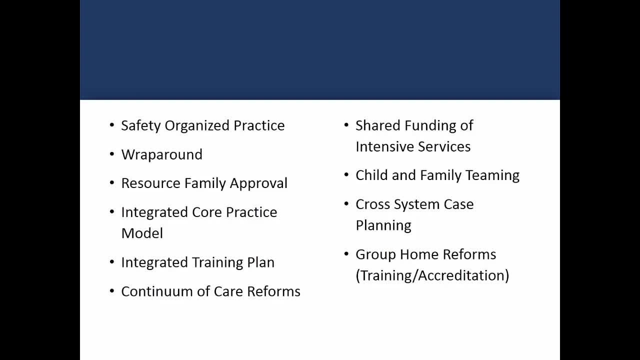 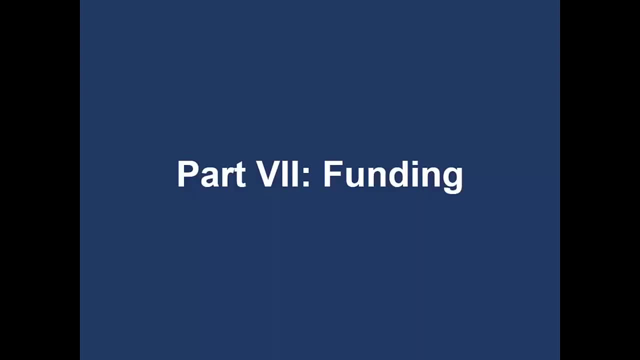 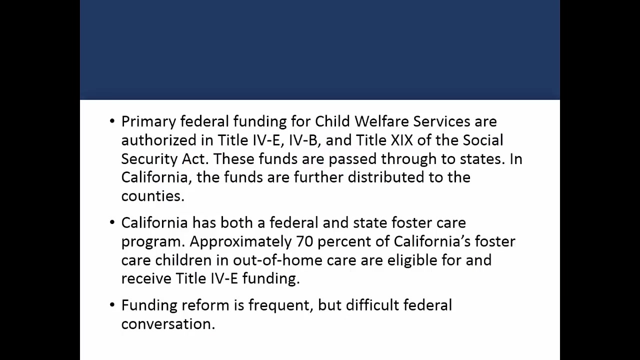 all service sectors work with families in a culturally responsive, family centered and strength based manner. California will be the first state in the country to have a fully system-wide core practice model. It takes an integrated and shared approach to funding child welfare services. Let's take a look at some of those processes and functions. The 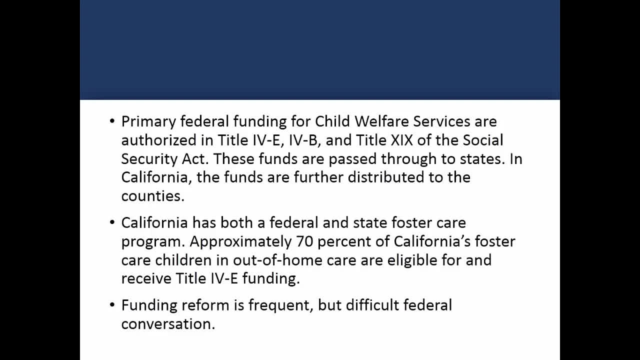 federal aid to families with dependent children. foster care program is a part of what's known as title 4e funding, which pay for placement for the board and care services that foster youth need. Foster children are also categorically eligible for medical, as we've mentioned children who do not meet the eligibility. 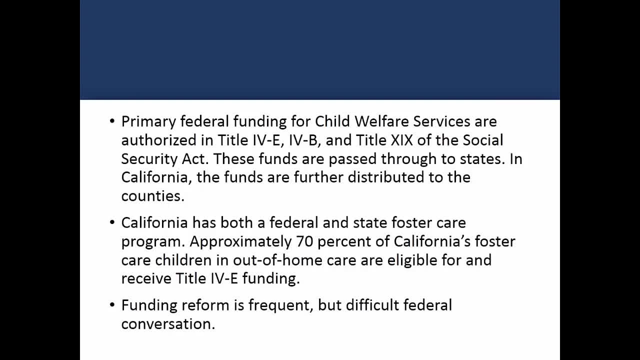 criteria for federal foster benefits are eligible for assistance under the state foster care program or the CalWORKs program if they're placed with a relative. the federal system which funds foster care is now more than 20 years old and badly in need of reforms, but consensus has proven challenging for